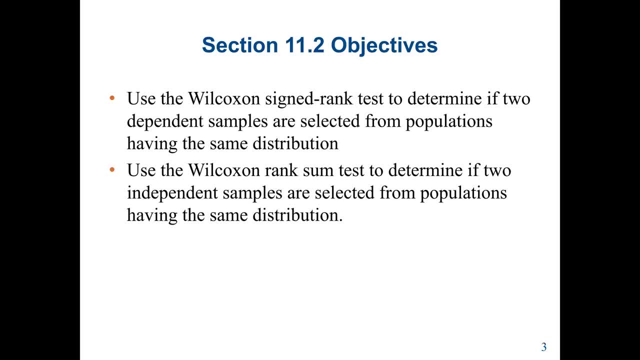 again we discussed in the previous lectures is that it wastes information. It's wasted information because the sign test merely counts the number of positive or negative signs in a pair differences experiment and also ignores the magnitude of the differences. But the recursive sign test is a parametric technique which can be used to 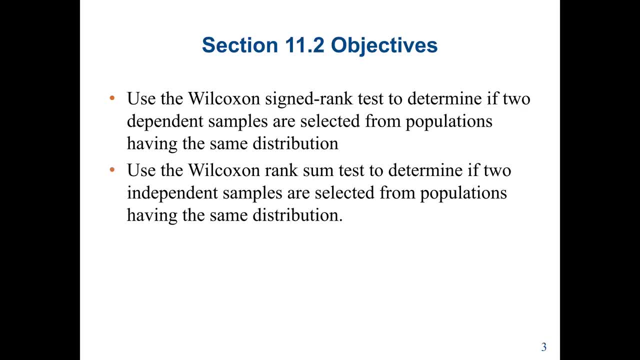 evaluate a pair difference experiment. This test is designed to detect again populations whose centers are shifted to the right or to the left of each other. But, as with the sign test, no distributional assumption is required. However, the pairs of data must have been selected. 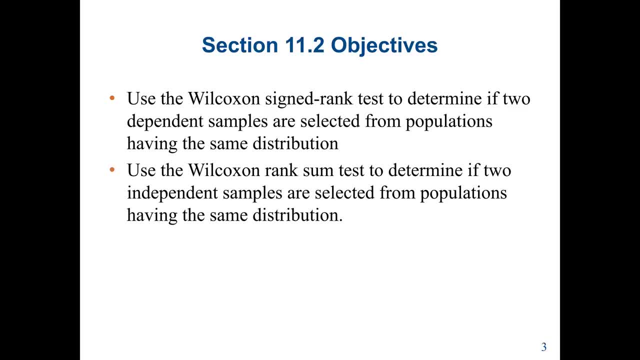 in a random function And it must be possible to run the differences. This is, again, the main condition of a sign test. So again, the disadvantage of a sign test is that it wastes information, because the sign test merely counts the number of positive or negative signs in a pair difference experiment and ignores 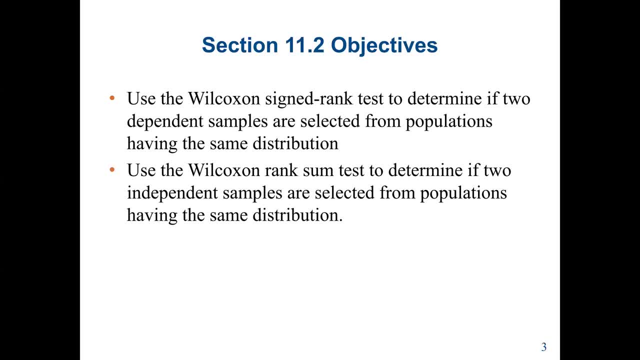 the magnitude of the differences. The advantage of recurrence is that the pair difference experiments are not going to ignore the magnitude of the differences. The advantage of a sign test is that it does not ignore the magnitude of the differences, but it does not take the magnitude. 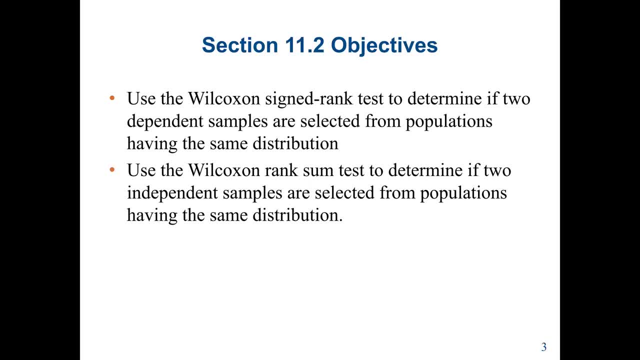 directly into account. Instead, the ranks of the data are analyzed. So again, that's the main difference between the pair difference experiment and the pair difference experiment. So again, that's the main difference between the pair difference experiment and the pair difference experiment. 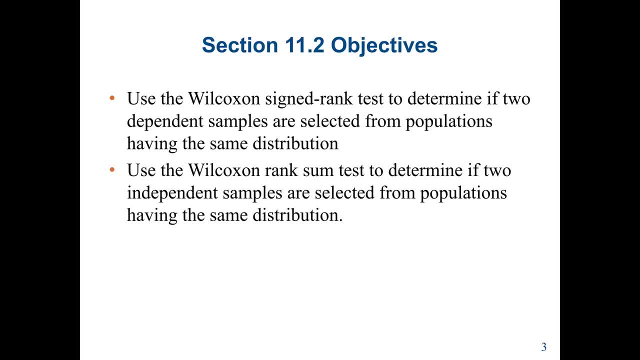 So again, that's the main difference between the pair difference experiment and the pair difference experiment. So here the advantage of a sign test is that recurrence and disadvantage are not considered in this praticamente common testing format. This is the�� that we talked about, that these patterns vary depending on what kind of 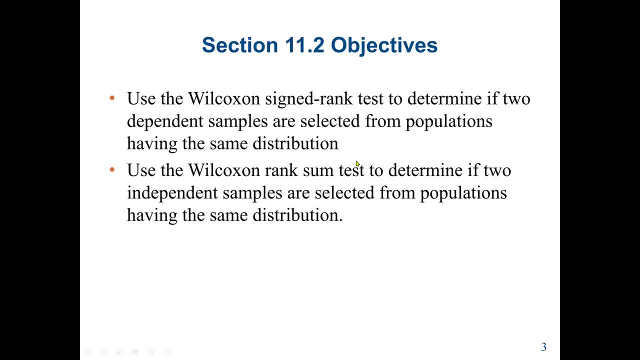 model we are using. so Tunisia helps to then indicate their Fill standards and, as we also saw in the before stool Renovation, survive and we are going to out received some of these results. So again, the advantage and disadvantage are Away from the milk test. 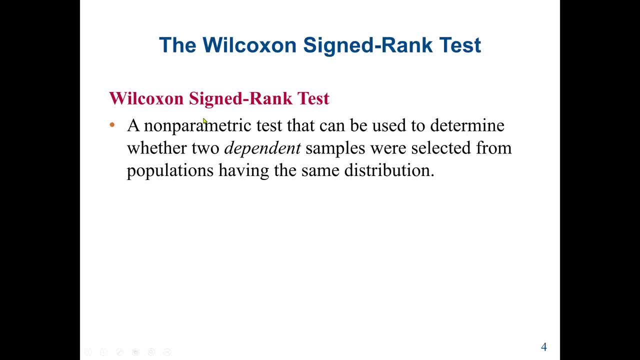 So here I've put the terms only in the shared list, Okay. Wilkerson sign rank test is a non-parametric test that can be used to determine whether two dependent samples were selected from population having the same distribution And, unlike the sign test, it will consider the magnitude or size of the data entries. This is the advantage, again with the Wilkerson sign rank test. 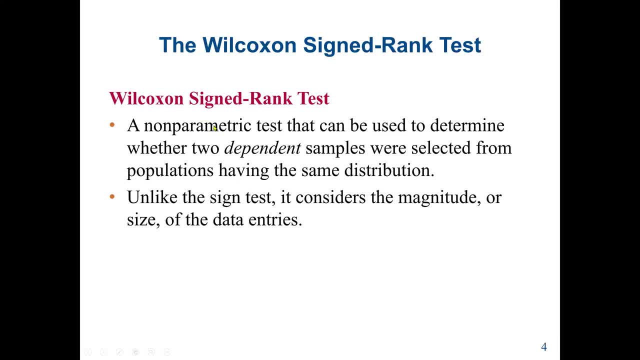 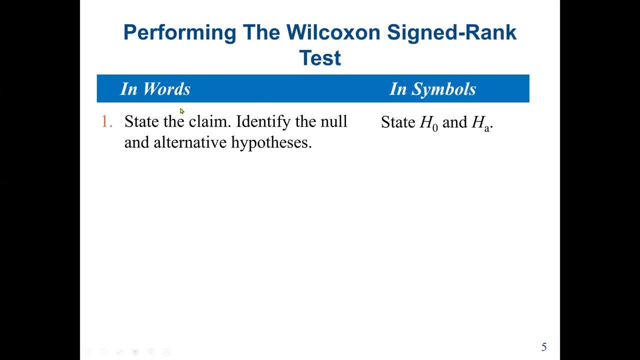 Our previous sign test, the magnitude, again is ignored. So let's go through the steps of performing the Wilkerson sign rank test In words again. this is also hypothesis testing. So first we need to state our claim, So we need to identify the null and also the alternative hypothesis. 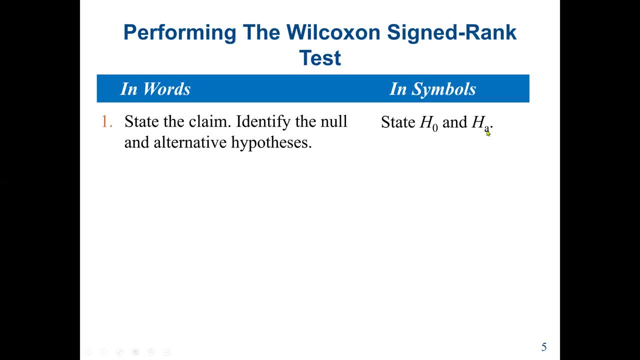 So we need to state the HO and HA, As we said in our previous lectures. always HO will be our claim and HA will go against the claim. Then we need to specify the level of significance, which is the number of samples that were selected. 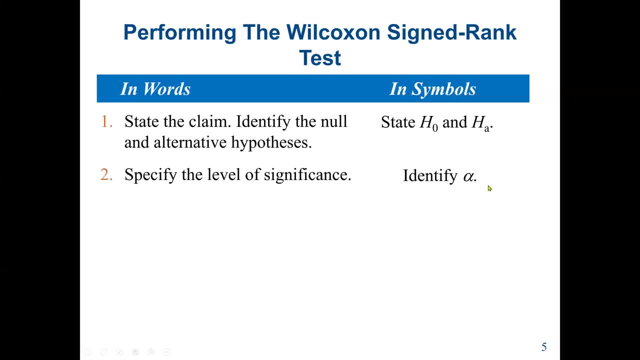 So we need to identify the alpha, The level of significance always is given to us. Then we need to determine the sample size, N, which is the number of pairs of data for which the difference is not zero. Remember, in the sign test, the same concept. 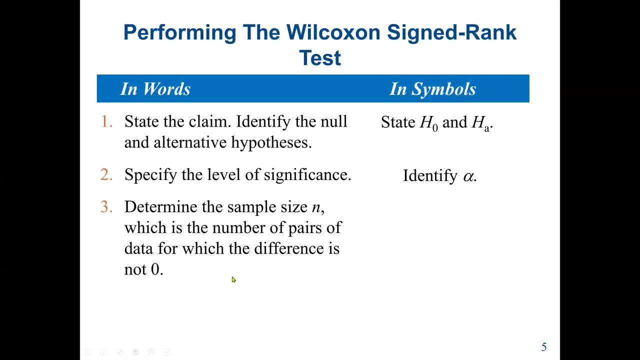 When the difference of the two pair data set is zero, which means the sample is the same, we ignore it. When one is less than the other, the left is less than the right, or let's say the first one is less than the second one, then we assign negative. 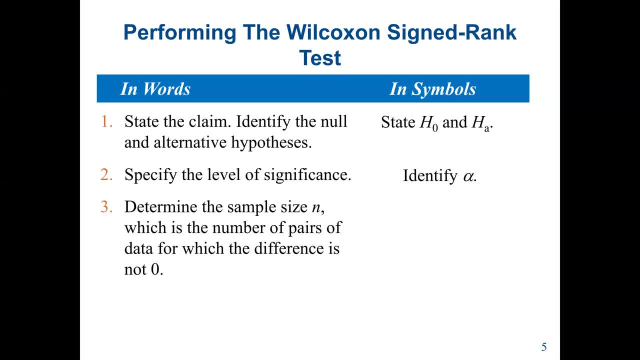 If the first one is greater than the second one, we assign positive. The same concept. here. we determine the sample size, which is the number of pairs of the data for which the difference, again, is not zero. Then, after that, we determine the critical value. 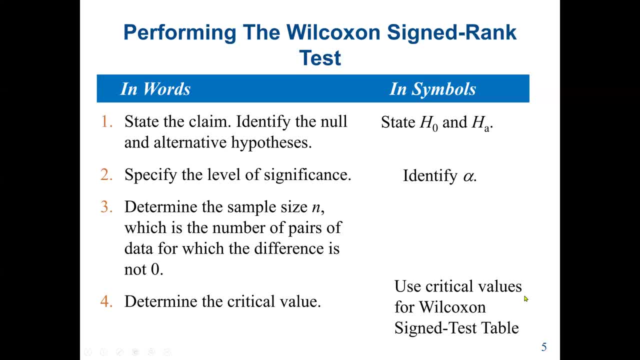 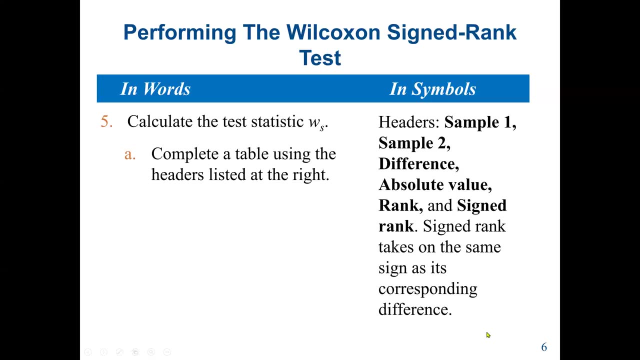 So the critical value, we're going to use the critical value for Wisconsin sign test table And we have a special table for, again, Wisconsin sign test. In order to use the table again, we need the alpha value, the level of significance. 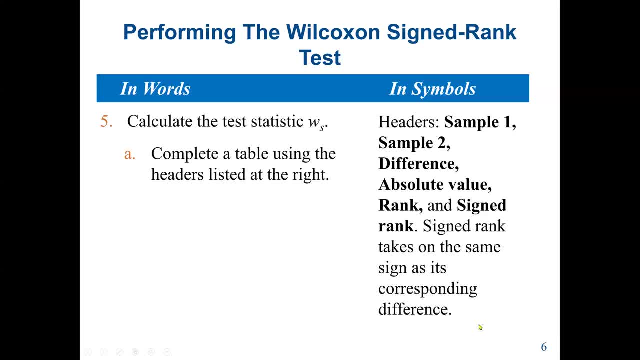 So after we get our critical value, we can now know the boundary between where we have to reject the HO or accept the HO. So next we need to calculate the test statistics. So we complete a table using the headers listed at the right. 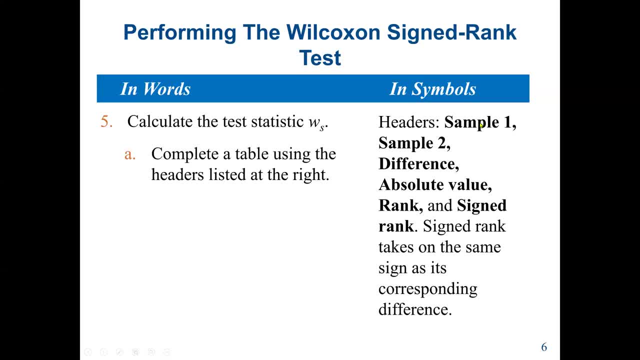 So our headers should be. we have two samples, So we have sample one, sample two, The differences of sample one and sample two. we have a difference column. Now if the value is negative, we look for the absolute value. We know, for example, if the difference is two, the absolute value will be two. 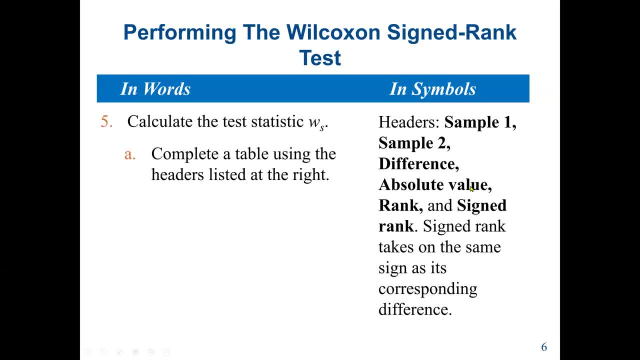 If the difference is negative two, the absolute value will be two. So first we have the sample, the first column, sample one. second column, sample two. The third column will be the difference of sample one, sample two values. Then the result we get, we find the absolute value of it, of the difference. 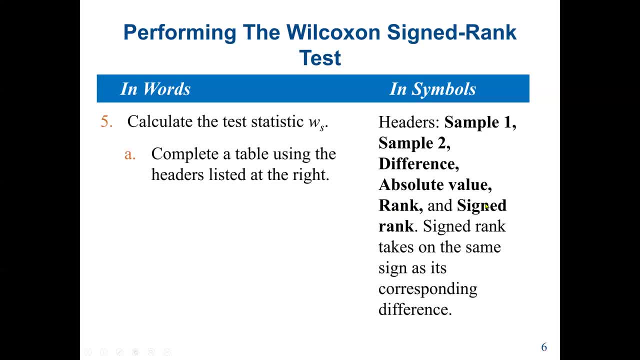 Then we rank it, Then we assign the sign rank. So here we say the sign rank takes on the same sign as this corresponding difference. So again, complete the table using the header listed at the right. Then we find the sum of the positive ranks and then the sum of the negative ranks. 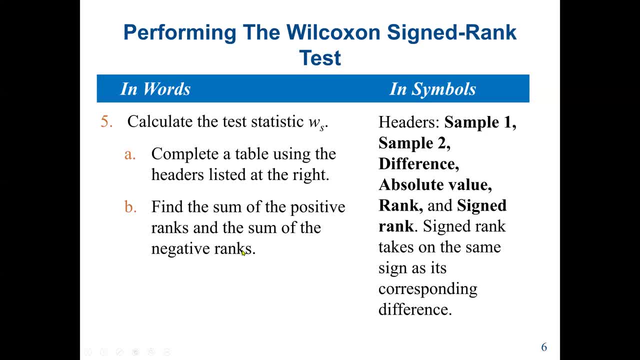 The same step as we did in the sign test. In the sign test, again, we have two groups. We find the differences. If the difference is zero, we ignore it. If it's positive value, we count positive. If it's negative value, we increase negative. 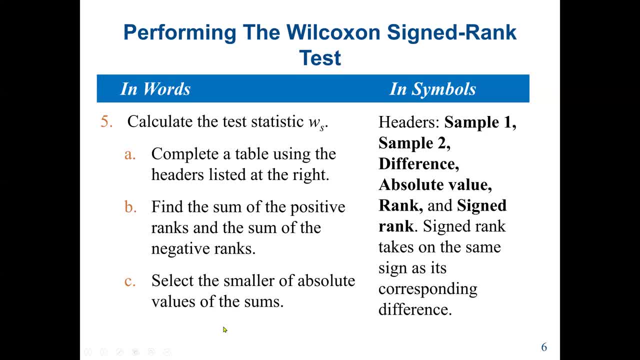 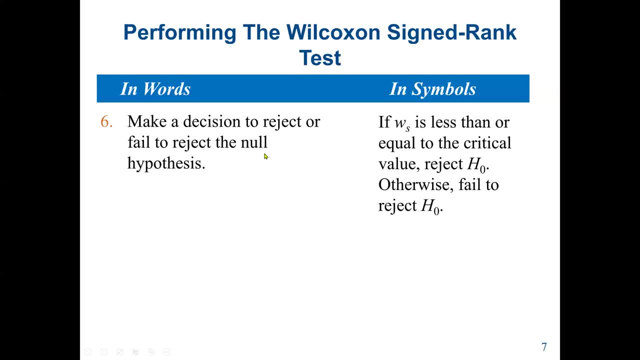 So next we select the smaller of the absolute values of the same sums. Then, step six, we make a decision to reject or fail to reject the null hypothesis, which is the HO. So here we say: if our WS, which is our test statistic, is less than or equal to the critical value, 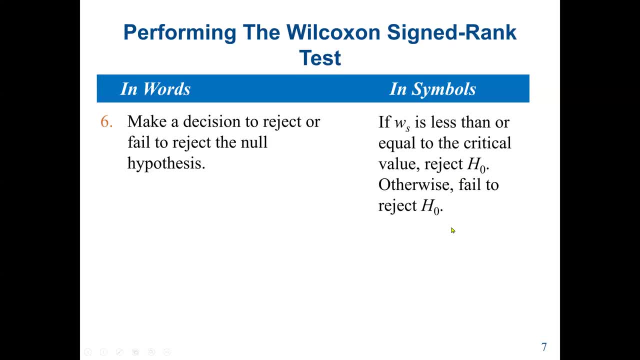 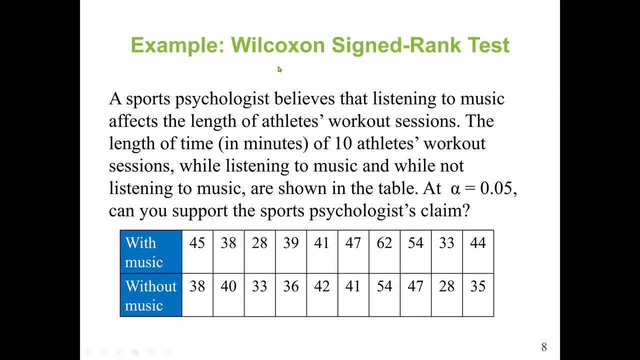 then we are going to reject HO. Otherwise we fail to reject HO, Then we interpret the decision in the context of the original query. So I think the example here may help us. So this is an example of a reconsent sign rank test. 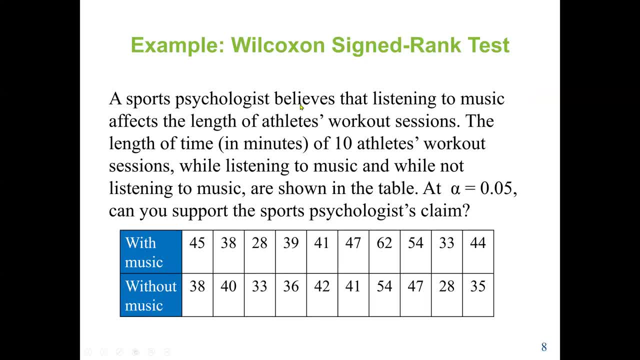 As we said earlier, the reconsent sign rank test is normally used again to test if two data, two samples, came from the same population distribution. The distribution of the populations are the same. So here let's see our example here. A sports psychologist believes that listening to music affects the length of athletics workout sessions. 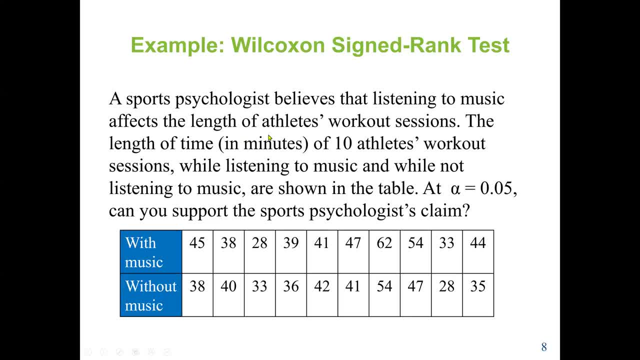 Again, listening to music affects the length of athletics workout sessions, The length of times in minutes of 10 athletics workout sessions while listening to music and while not listening to music. So this is again dependent sample, Dependent sample or dependent data because we are using the same athletics. 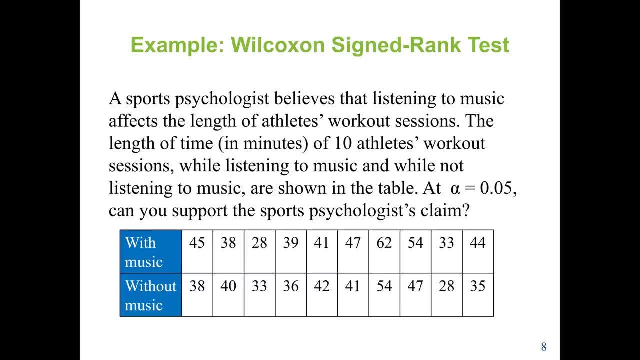 Now if we have athletics A in group A listening to music- group B didn't listen to music- they are different people- then that would be independent sample. So when we read the question again, the reason why I want us to understand dependent sample: 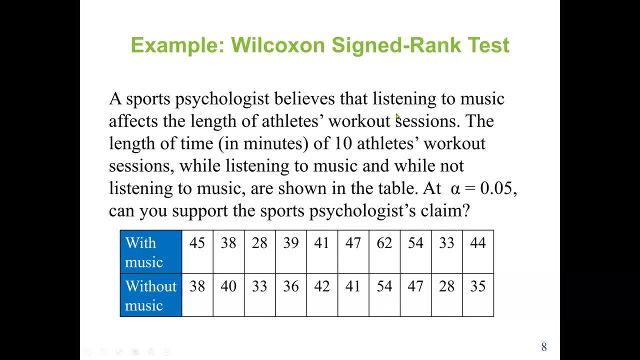 because again, Wisconsin sign rank test, we test it on two dependent, two dependent variables, not two independent, two dependent from the objective. So here we see: a sports psychologist believes that listening to music affects the length of athletics workout sessions, The length of time in minutes of 10 athletics workout sessions while listening to music and while not listening to music. 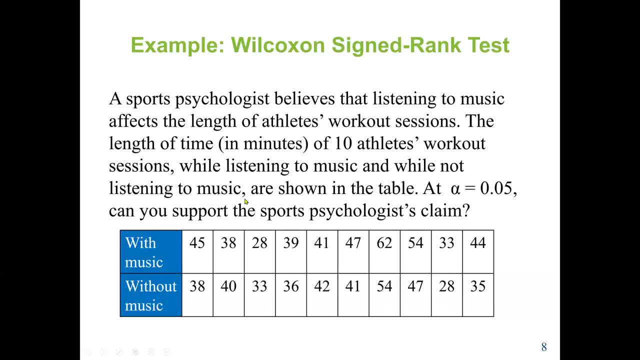 The length of time in minutes of 10 athletics workout sessions while listening to music and while not listening to music. So it's the same group of athletics, 10 of them. So this is again dependent sample as shown in the table. The alpha level is given to us to be 0.05.. 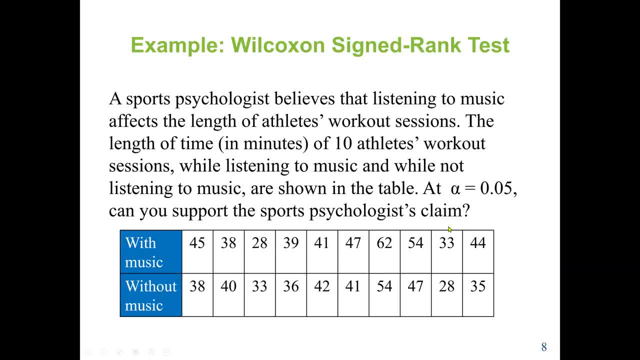 Now, can we support the sports psychologist claim? The sports psychologist claim is the beginning of the sentences. here the question: The sports psychologist believed that listening to music affects the length of athletics workout sessions. The sports psychologist believed that listening to music affects the length of athletics workout sessions. 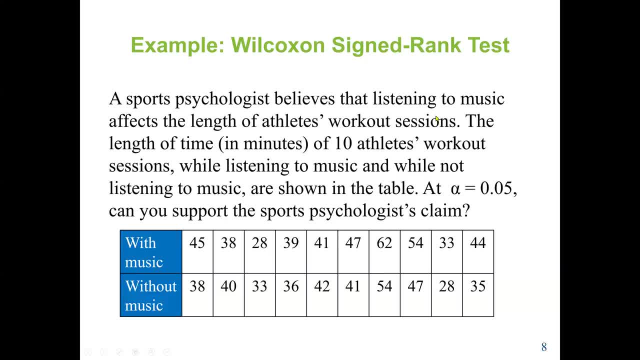 So does it affect or does not affect? So these are the sessions. We have 10 athletics, Again the same person. When he's listening to music, it's 45 minutes. Without music, it's 38.. The next athletics listen to music: 38.. 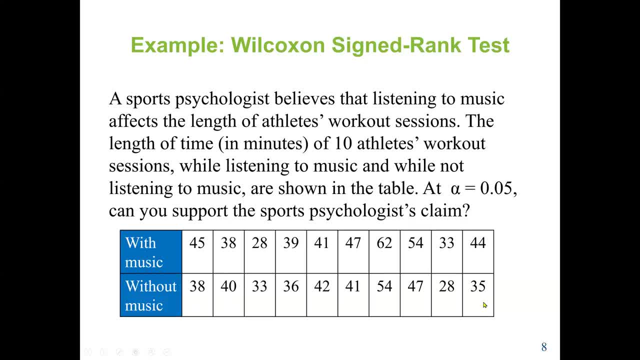 Without listening to music 40.. Without listening to music 40 again. So by looking at this question we can use that we cautious soundind wrong test. The reason why? Two things. This is two samples pair. not only that, but they also dependent. 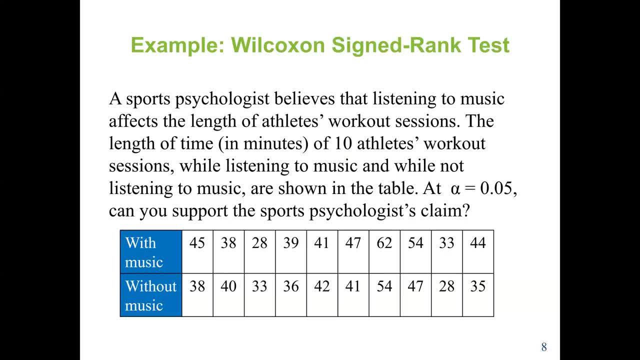 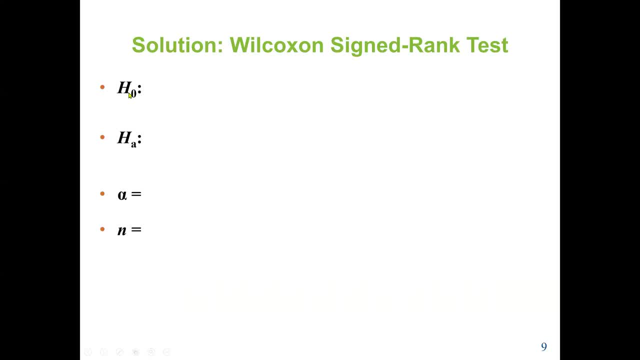 Most important thing is two dependent samples. So let's go step-by-step, as we went through the steps already. First we need to state our claim. So we have our HONHA HOSA, Our University of Wisconsin. So we say there's no difference in the length of the athletics workout section, which is 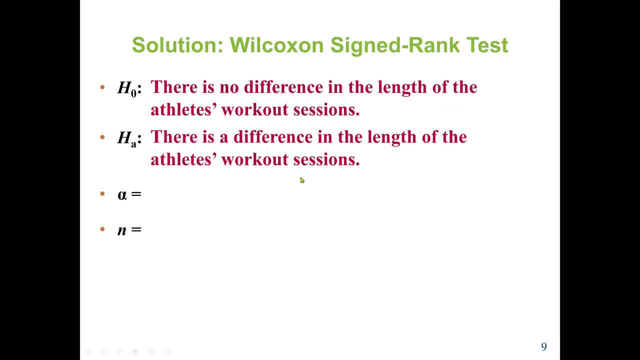 equal against it. So there's a difference in the length of the athletics workout sections. Alpha is given to us to be 0.05.. So we have the alpha value 0.05 and it's a two-tailed test. The reason why it's a two-tailed test: we can see difference or no difference. 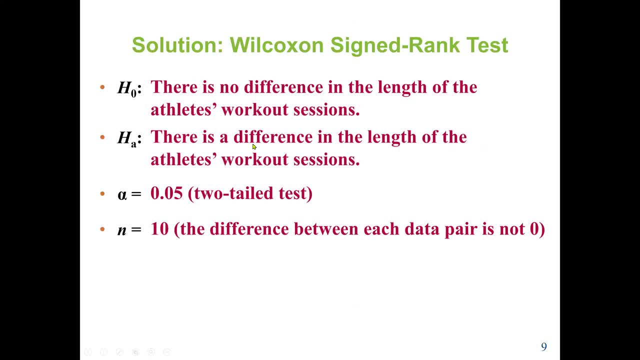 So it's equal or not equal. There's no greater or less, either there's no difference or there's difference. So this means it's a two-tailed test. And then the sample size, and we have 10 athletics from the same dependent, the same sample. 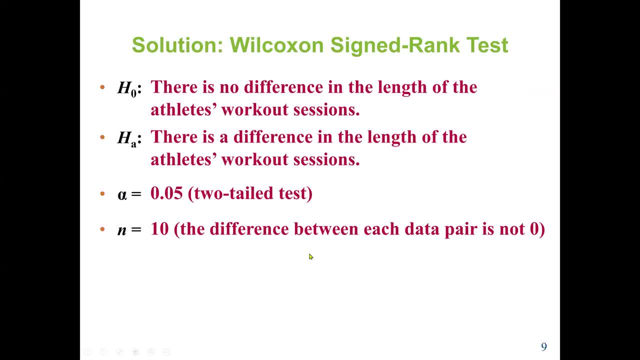 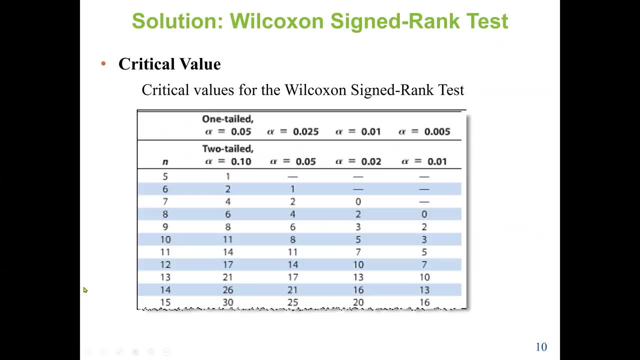 They are listening to music and they are not listening to. So here we say: the difference between each data pair is not 0.10.. So here we know that this is again the table we are going to use to find the critical value for Wisconsin SignWrong test. 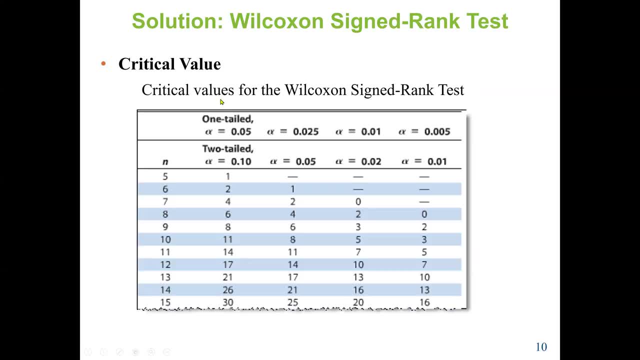 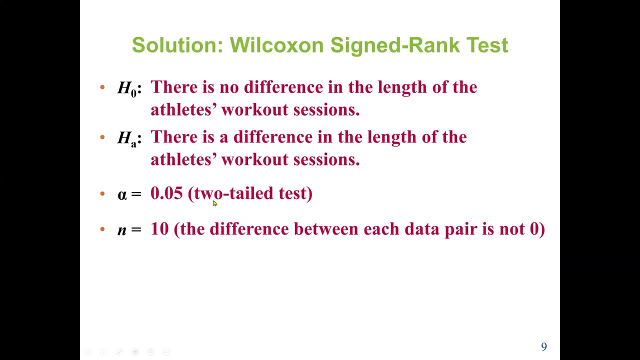 Again, that's the name of the table: critical values for the Wisconsin SignWrong test, And the answer here will be eight. The reason why, again, let's go back. We saw the alpha level is 0.05,, it's a two-tailed test and it's 10, because when we see our 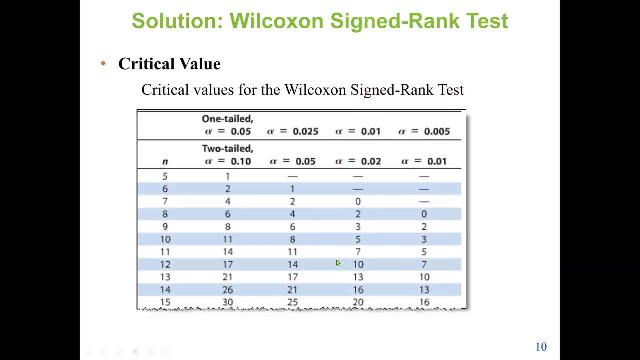 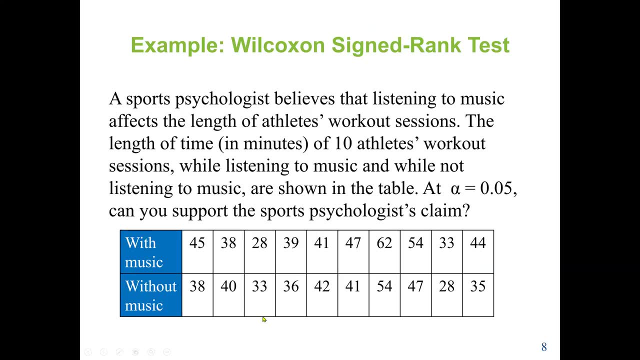 data. there's no zero. Let's go back to the data First, then we look at the results. So when we look at the data here, there's no any data set that the value is zero. So it's the same: 10 athletics with music, how long it takes with that music, how long. 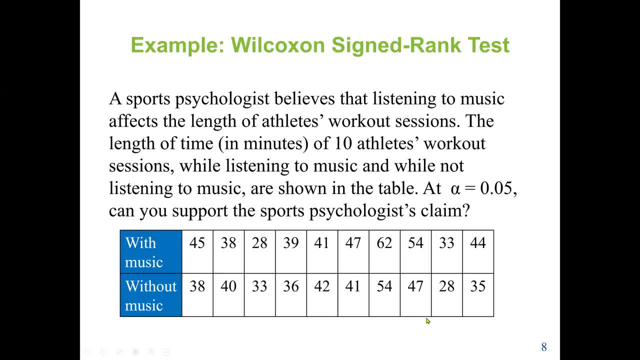 it takes And the time for all the 10 athletics is the same. I mean the time. there's no differences, There's always. I mean there's differences, There's not the same two values. So, for example, the first athletics 45, 38,, second, 38,, 40,, 28,, 33,, 39.. 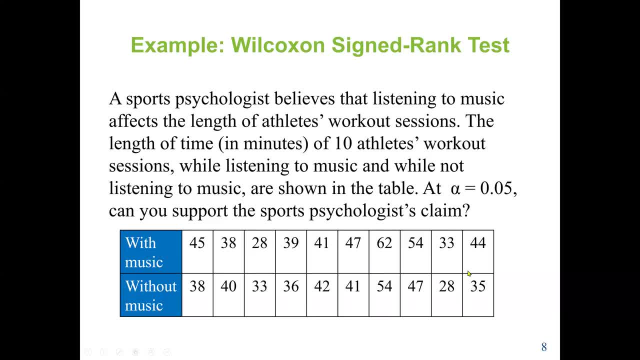 So all the minutes that we get, the length of the sessions with music and without music. there's a difference in time. We don't have the same time. What I mean we don't have the same time. Let's say, the last athletics with music was 44, without music was also 44.. 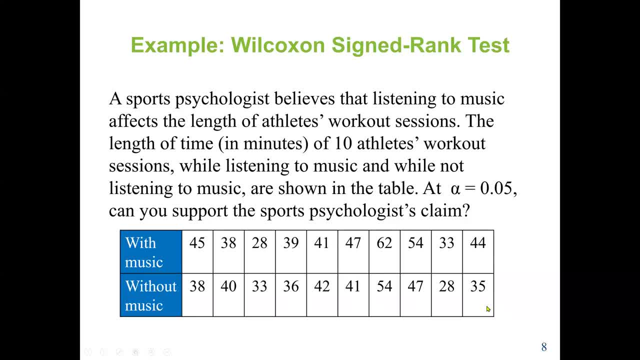 So if that's the case, the sample will be nine, not 10.. So remember: in the steps we said: if the difference is zero we don't count it. So here we count everything, because the differences of all the 10 athletics is not zero. 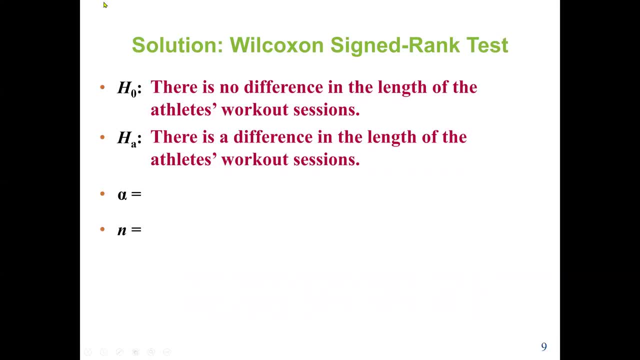 So we count it. So that's why, again, again, the first step, we say this: our HA and HA, we have the alpha And the reason why we have 10, there's the differences between each data pair is not zero. 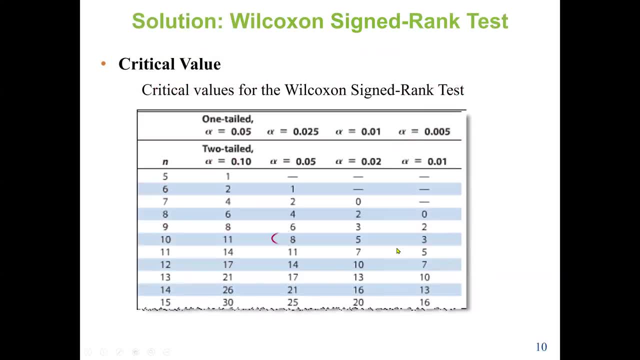 So now, since I know the N to be 10, so I'll go to the N is 10.. And also, I know the alpha is 0.05,. two tail, two tail, not one tail, two tail. So two tail, 0.05 and N, that will give me eight. 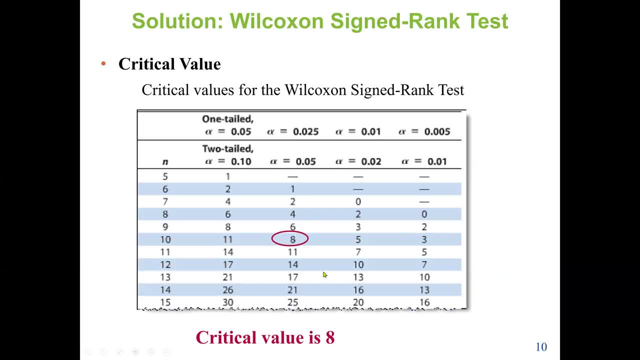 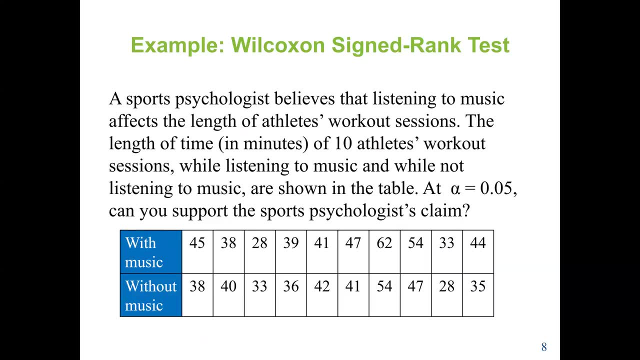 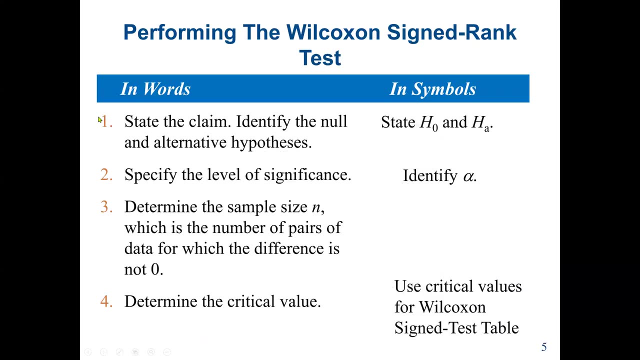 So this means my critical value is eight. Again, I'll go through this example one more time from beginning. Okay, And also let's go through the steps one more time. So here we are, performing the Wisconsin sign rank test. So the first step again is to state our claim, identify the null and also the alternative. 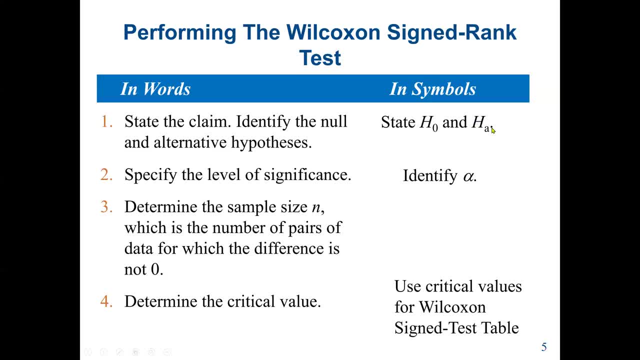 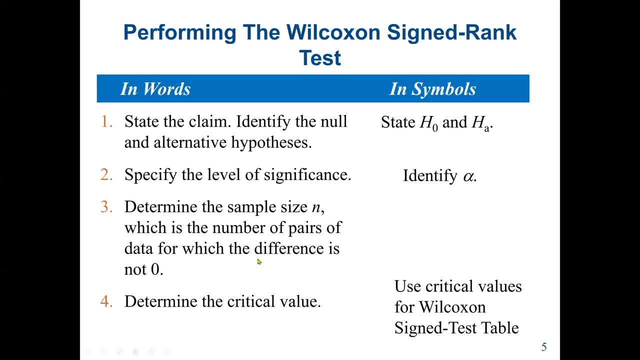 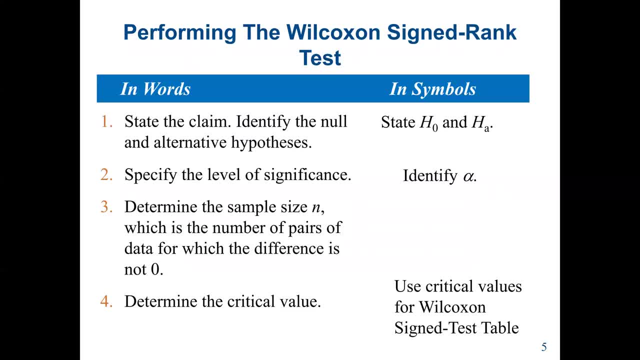 Yeah, we have 10 athletics. The difference of the session, the training session, with listen to music and without listen to music, The difference of all of them is not zero. So that's why we use N equal to 10, because all of them. 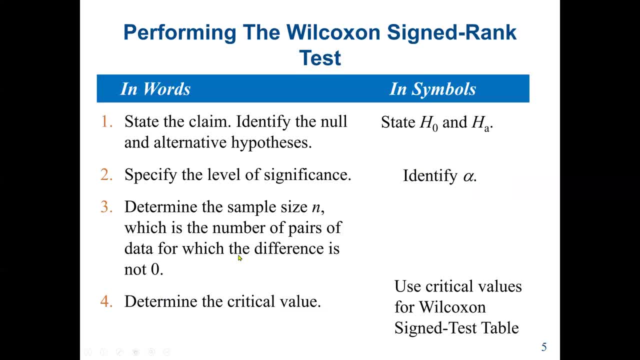 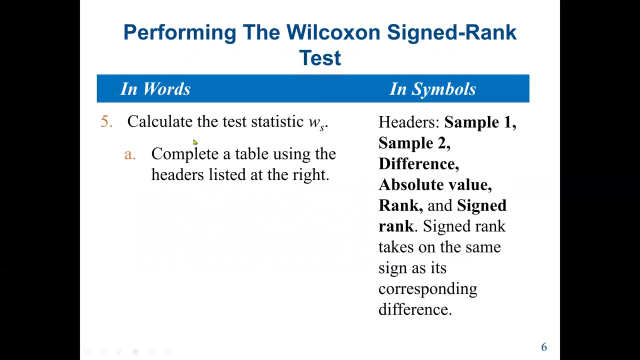 So if we know this, we know the alpha level, we know the sample size N, where the difference of the values is not zero, Then we can go to the Wisconsin table to determine the critical value. Then we determine the critical value. So after we determine the critical value, now we calculate for the test statistics. 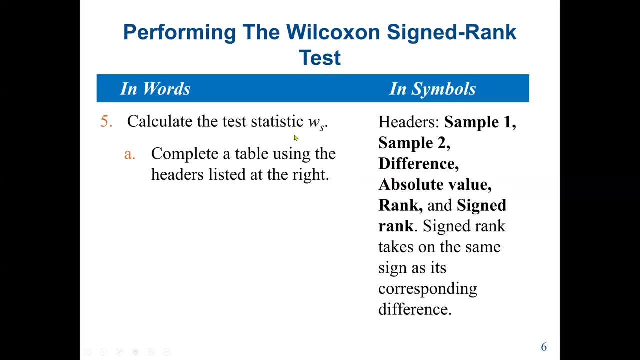 which is the BUS. In order to do this, we have to set our table. We have sample one as our first column, sample two, then we find the differences of sample one and sample two, Then we find the absolute value from the differences, Then we rank, then we assign. 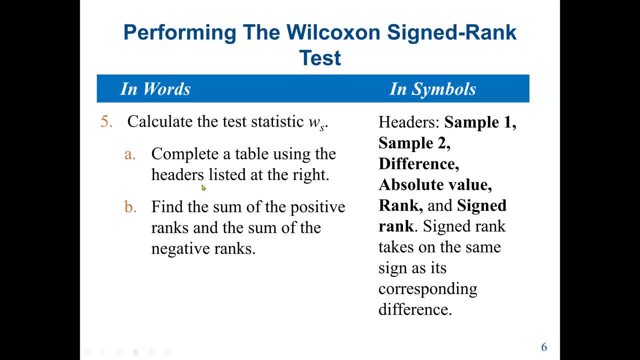 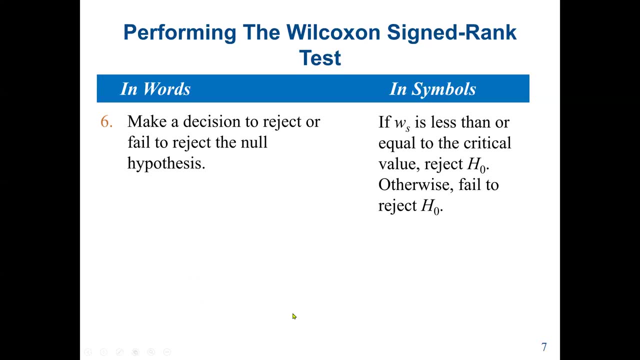 ranking. So we complete the table using the headers listed at the right. Then we can find the sum of the positive ranks and the sum of the negative ranks. Then we select the smaller of the absolute values of the sums. From there we can make our decision. 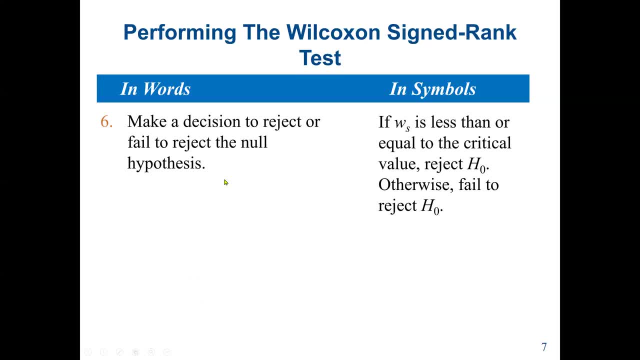 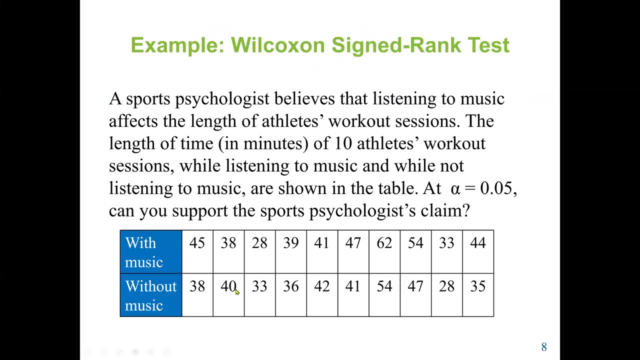 So we make a decision: Either we are going to reject or we are going to fail to reject the HO. Then we're going to interpret the decision in the context of the original claim. So this is the example again. So yeah, we said again: sports psychologists believe that listening to music affects the length. 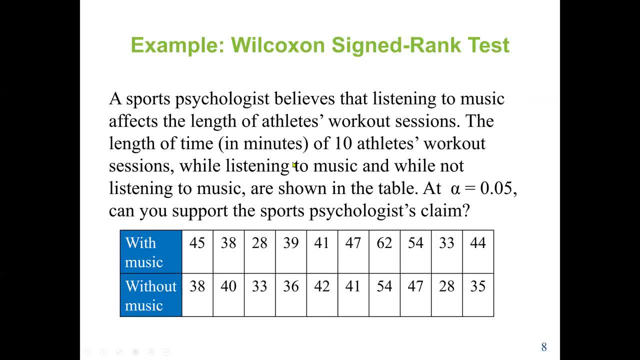 of the athletic's workout session. The length of time in minutes of 10 athletes' workout workout session- why listen to music and why not listen to music- are shown in the table below and at alpha 0.05.. Now can you support the sports psychology screen? Yeah, we have. 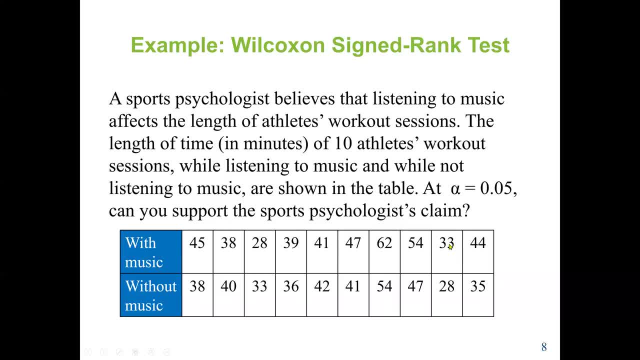 with music. this is the time they spend in the session workout section Without music. they give us the time in minutes they spend in their workout session. Now, when we look at all the 10 athletics, there's no difference. that equal to zero. So our n equal to 10,. 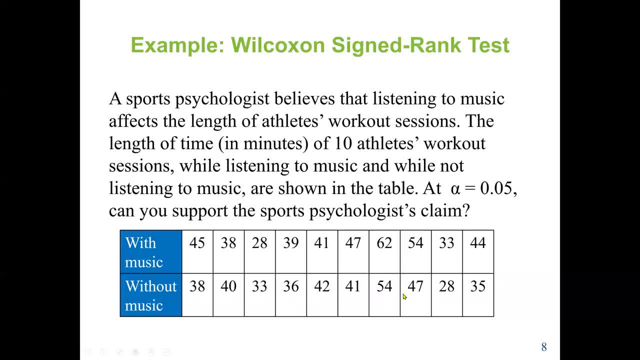 the whole 10 of them, The ones that equal to zero, we ignore it. So let's say, if we have 44 and 44 at the last, we are going to remove it. So our n will be nine. So we: 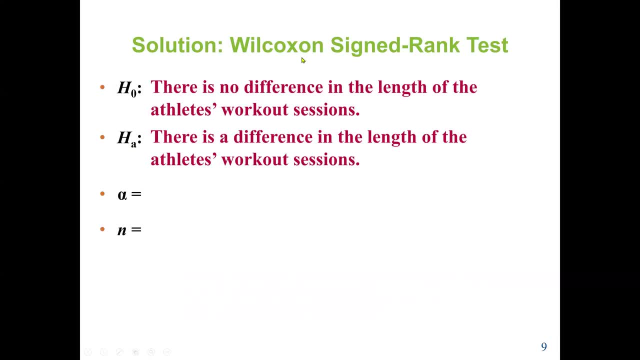 start with stating our claims. We know here we are looking for the differences in length of athletics workout session. So HO said it's there's no difference. HO said there's a difference. Alpha is already given to be 0.05 and n is 10 because the difference between each data pair is not zero. Then from there, 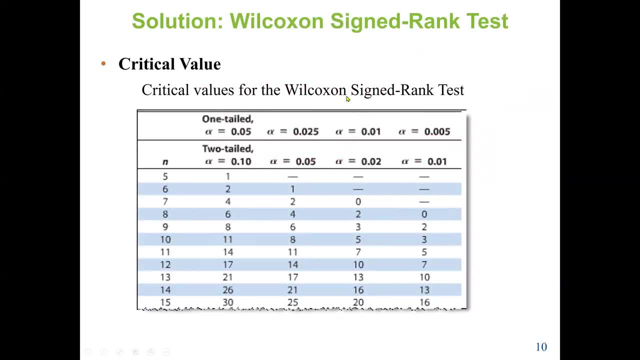 we go to the critical values, for we call it the sign-rank test. Now we look for: n is 10.. We have two tails. Alpha is 0.05.. So it will be this column here: Alpha is 0.05.. 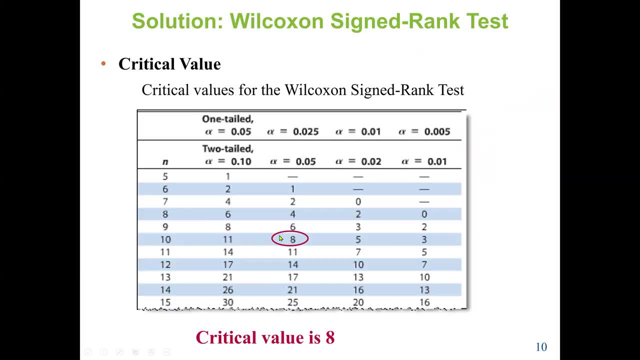 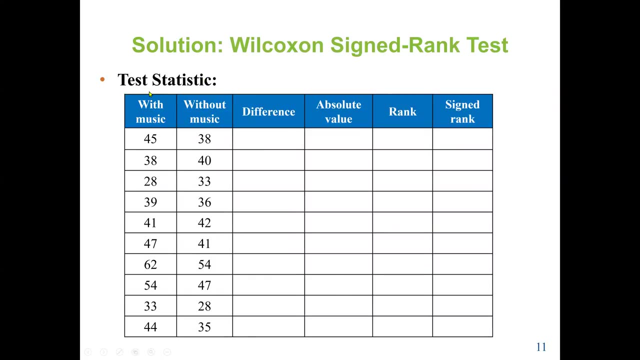 And the value is eight because n is 10 on the row 10.. And then two tails, 0.05 is eight. So if we know this, the next is to calculate the test statistics. The test statistics: they say we should arrange our table So we have our data. set is about section workout. 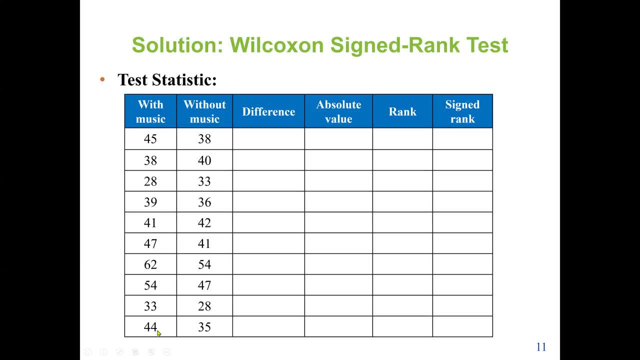 section with music. So these are the 10 values. is in minutes for the athletics, then with that music. this is it. so with these two we can find our differences. so the difference between 45 and 38 is 7. 38 minus 40 is negative 2, 28 minus 33. 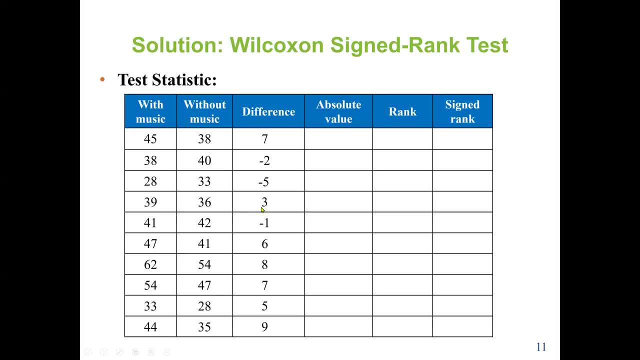 negative: 5, 39 minus 36 is 3, 41 minus 42 is minus 1, all the way to the end. so last is 44 minus 39, which is 9.. so now we're going to find the absolute value of the differences. so everything. 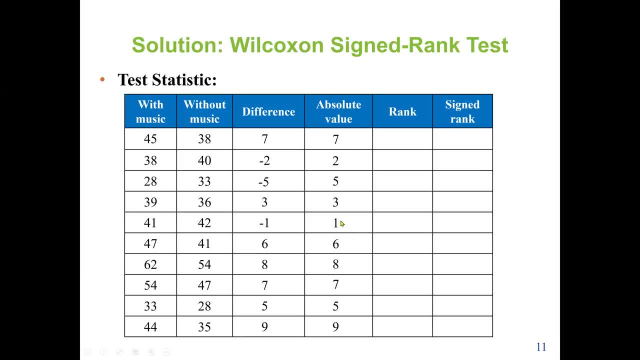 will be positive. now the same value. so negative 1 will be positive 1, negative 5 will be positive 5.. so when we get this data now, we can do our ranking now. so we look for the lowest. so the lowest is one, so first round one. the next diff absolute value: smallest is two. 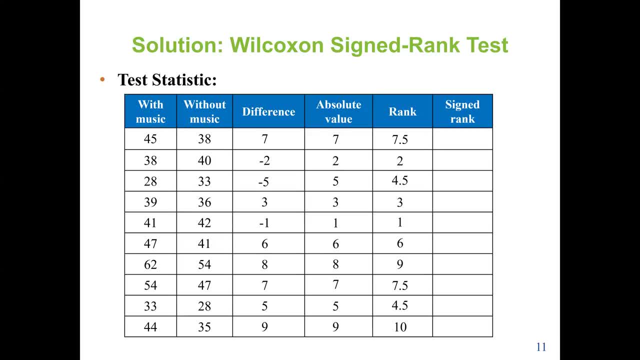 three. we don't have no four, but we have five. since we have two fives, we use 4.5, 4.5. then we move to six. six is six, then seven. maybe we have two sevens. there is also 7.5. it means we have two seven. 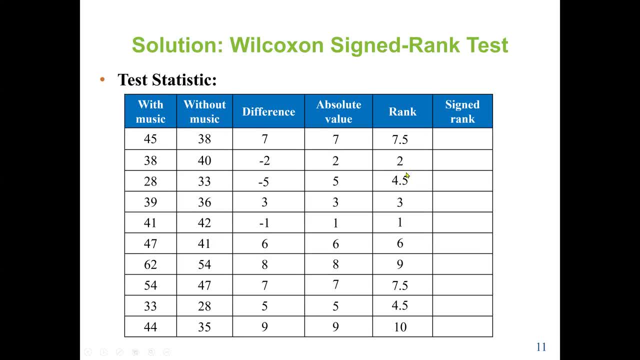 so we have one seven here, one seven here, so both of them will be 7.5- 7.5. then we have eight, then we have nine, and then we finish. so we rank them then. now we go to the next step, which will be our sign round. 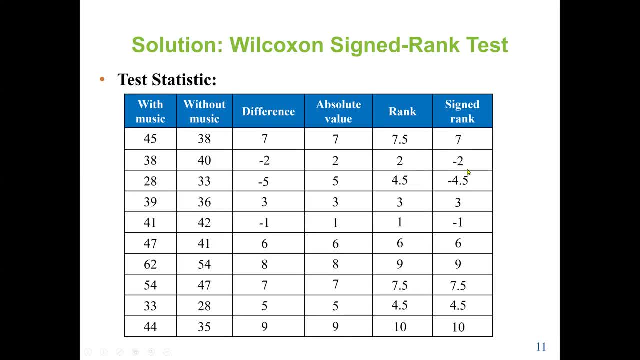 uh, here we have 7.57 and remember the difference is negative. so negative two. we also. we have negative 4.5 because the two negative. we have three: negative one, six, eight and nine, 7.5, everything is positive. so 7.5, then for city, 4.5 and then positive 10.. 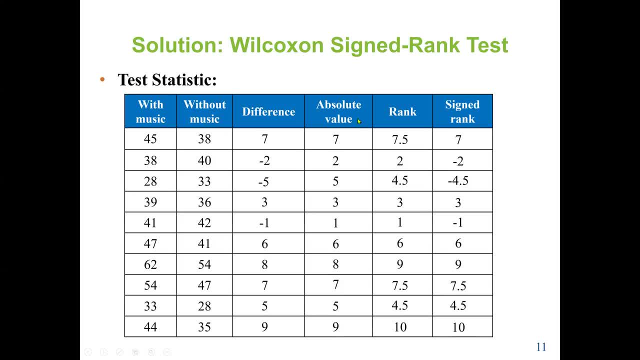 so this is our sign log, which is why the test is called we constant sign round test. so we are the first two columns will be given to us because we have a pair of dependent sample. we find the differences, then we find the absolute value, then we rank it. we rank it from the lowest to 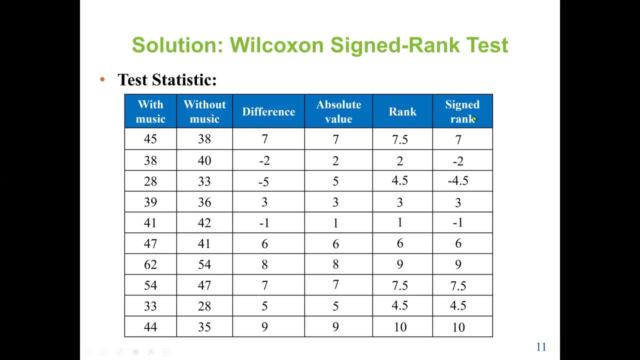 be first, Then we sign rank. it sign rank it depends if we have a negative or positive in the difference, negative or positive. So you can see, here we have one, one which is one. rank is one is the lowest one, but it was, the original was negative one. so we assign negative one as our sign rank. 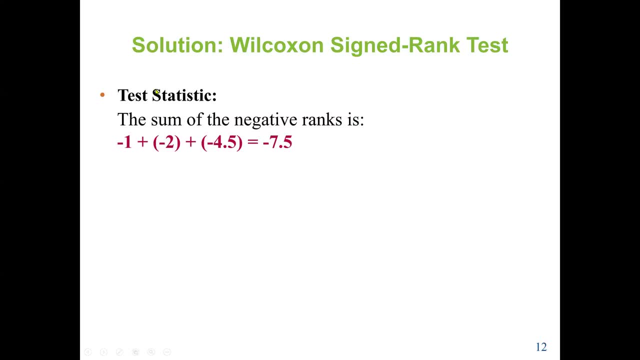 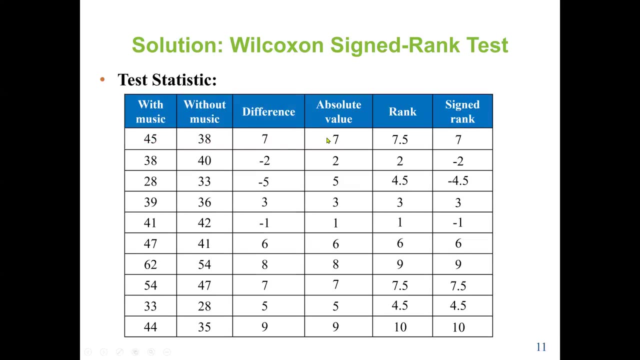 So from here we can find our test statistics. So the test statistics will be the sum of the negative ranks. So when we look we have to take the lowest and we can see that the positive is too many: one, two, three, four, five more than six. So when we look at the steps we take, 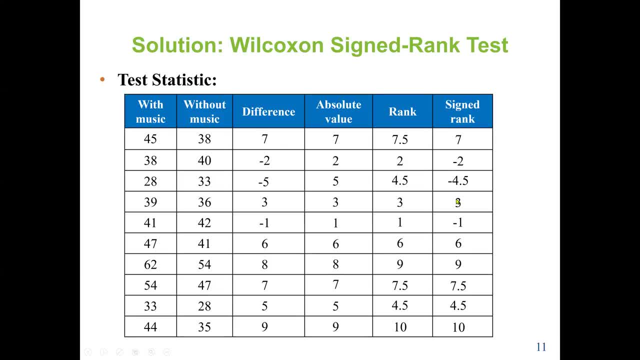 it can be positive or negative for the lowest items. So the lowest is negative. we have three negative. the highest is positive. we are seven positive. So we find the sum of the lowest is sign of positive or negative and the count shows that negative is only three, so it's lowest. 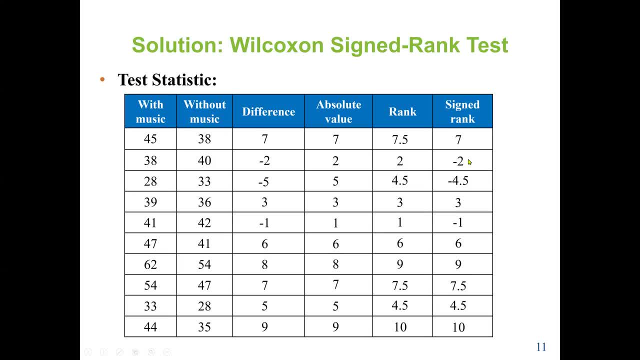 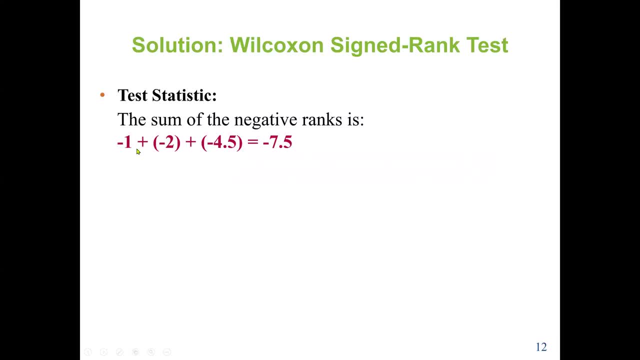 positive is seven. So we have negative two plus negative four point five plus negative one. and that's what we have here: negative two plus negative one plus negative four point five, which give us negative 7.5.. So this is our test statistics. Remember our critical value was eight from the table. 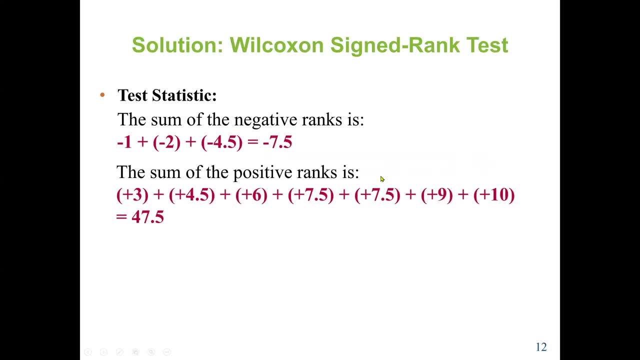 So the sum of the sum of the positive runs is 47.5. we had all the values of the signs. Then we have our WS now, which is our test statistics. We said it would be the small of the absolute value of these two sums, So it would be 7.5.. 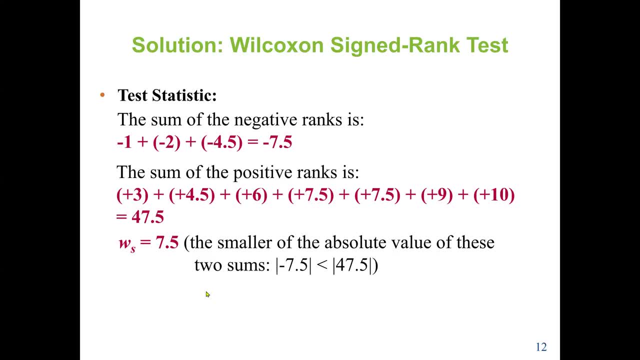 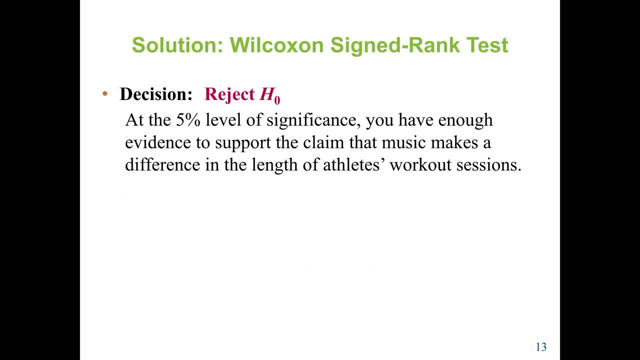 7.5 is our test statistics. We can make our decision that we are going to reject HO. The reason why we reject HO? because the critical value is greater than the test statistics. Critical value was 8.. The test statistics was 7.5. So we have to reject HO It. 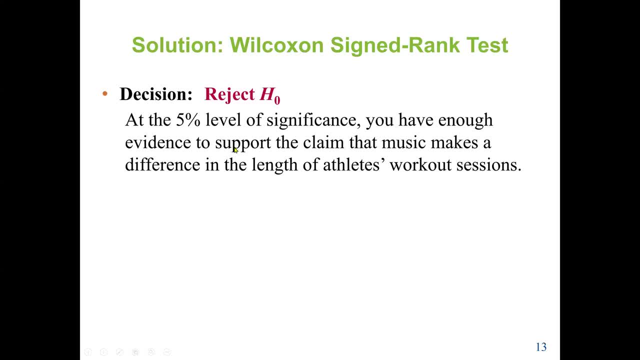 will go to the reject region. So we said: at 5% level of significance you have enough evidence to support a claim that music makes a difference in the length of athletics workout section. I think we can also see it in the table given to us, the two samples. 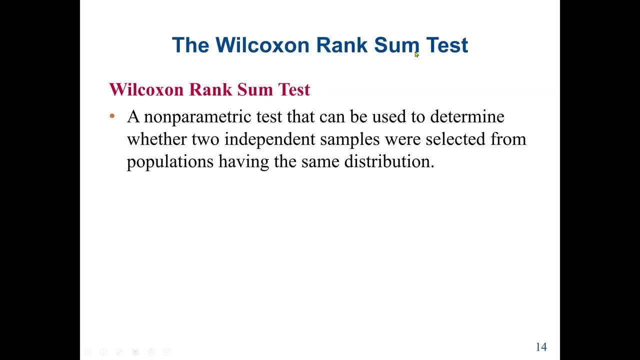 So next we move to the recursive rank sum test Also. a rank sum test is also a non-parametric test that can be used to determine whether two independent samples were selected from a population having the same distribution. So it's the same as a recursive sign round test. We say rank sum test. Previous was a sign round. 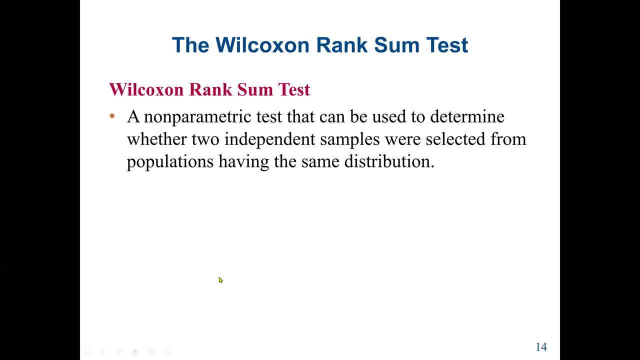 test. We are using these for the same purpose, But the steps are a little bit different. So here we say: the requirement for recursive rank sum test is that the sample size of both samples must be at least 10.. And also, M1 represents the size of the smaller sample and M2 represents the size of the larger. 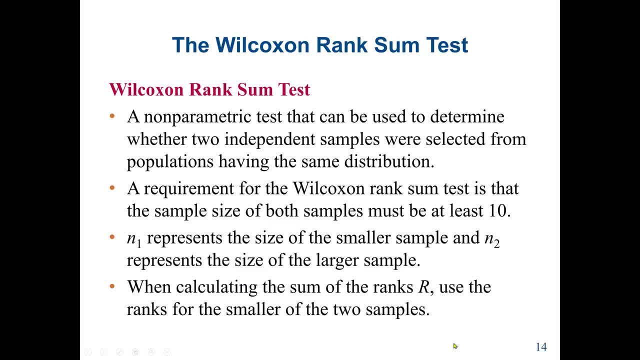 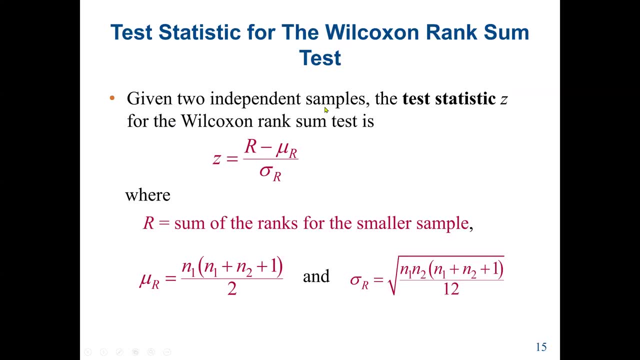 sample. So when calculating the sum of the ranks, use the ranks for the smaller of the two samples and the same concept as the previous. So this is the step, So giving two independent samples. the test statistic z for the recursive rank sum test. 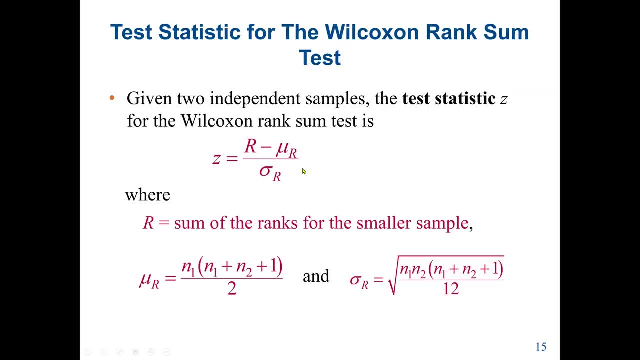 is z equal to r minus mu r over standard deviation r, And r is the sum of the ranks. for the smaller sample, The mu? r will give me M1 times N1 plus M2 plus 1 over 2.. And standard deviation r equals mu r over standard deviation r. 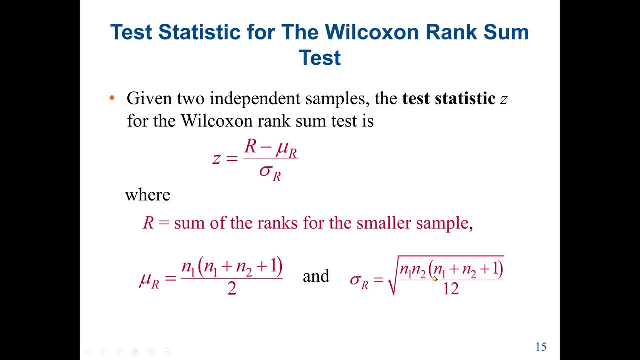 for R will be N1 times N2, N1 plus N2 plus 1, all divided by 12.. So the difference we are seeing here is that the formulas are different, but again, the steps are the same. So in our 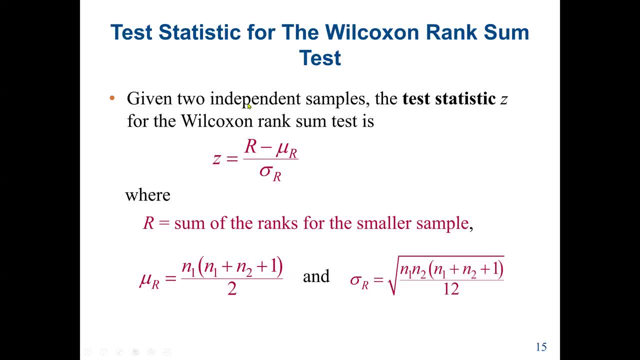 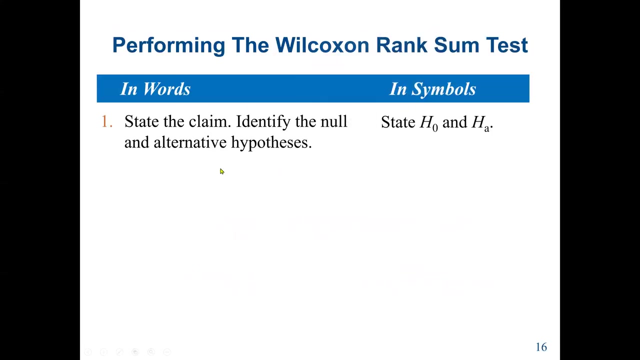 previous we used the critical value to find the recursive rank table, find the critical value for the. but here we are going to use the standard normal table because we find the Z. So our test statistics is using the standard normal table. we're looking for Z. 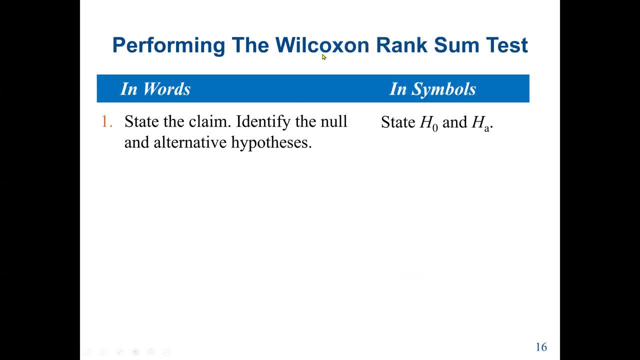 So let's follow the steps. Again, this is for recursive rank sum tests. It's different from recursive sum rank tests. It's totally different. So first we need to set our claim, HO and HA, Then we get our alpha: identify the level. 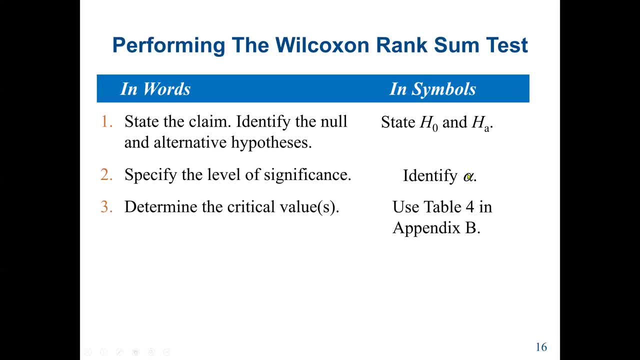 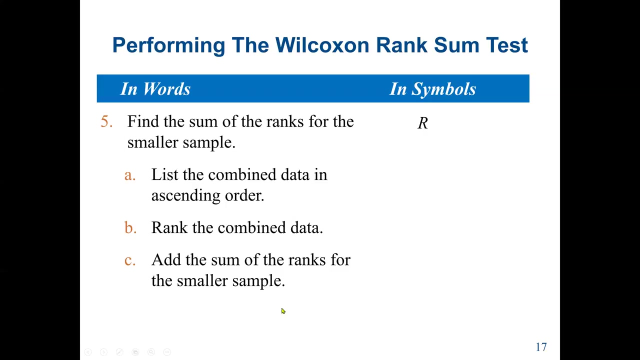 of significance, Then we, if I know the alpha, I can determine the critical value. Then we determine the sample size, Then we find the sum of the ranks for the smaller sample, Then we list the combined data and send the order rank, the combining data and had a sum of 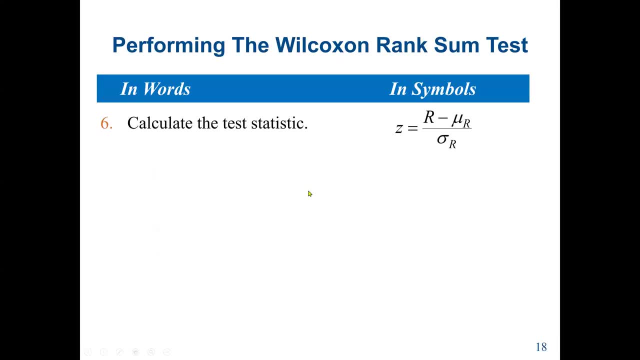 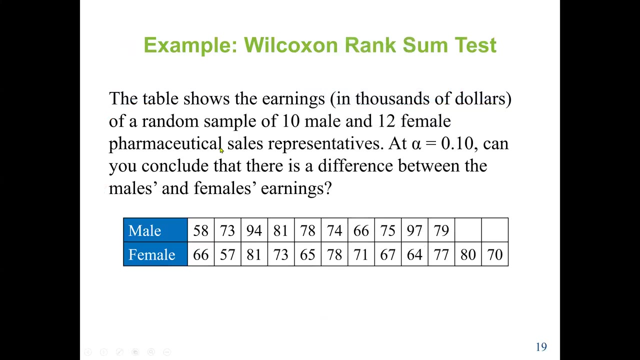 the ones for the smaller sample. Again, the best way to do this is solving the example. So we will see an example in a few seconds. So we calculate the test statistics, Then we make our decision whether to accept or reject HO. So this is a very good example. 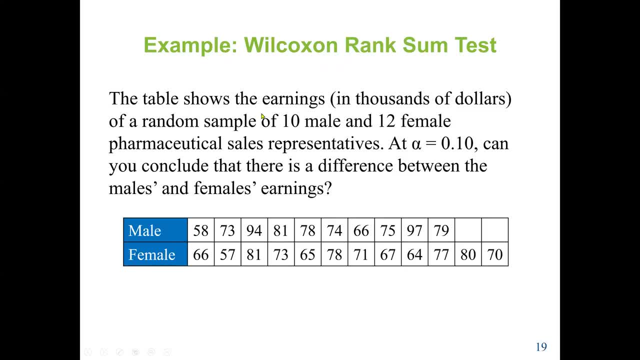 to explain the detail Here. we say we have a table- show the Hennies in thousands of dollars- Of a random sample of 10 male and 12 female Pharmaceutical cells, representatives at alpha equal to 0.10.. Can you conclude that there's a difference between the males and females? 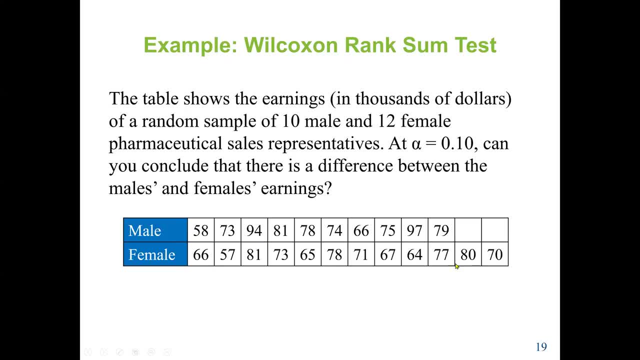 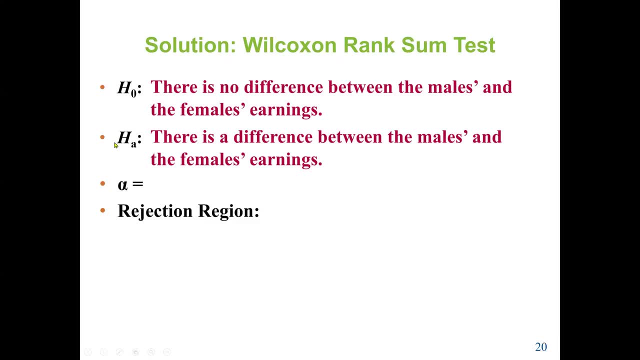 Hennies, So we can see the male Hennies and the female Hennies. So the first thing we state, our HO and HA HO is there's no difference between the males and also the females and Hennies, And alpha is given to us to be 0.10.. Since there's no difference, there's difference. 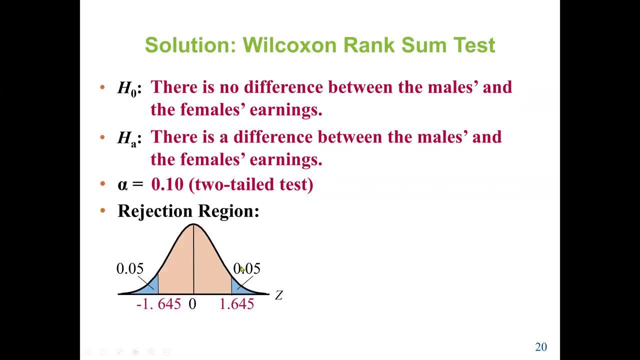 It should be a two way test. So we were able to find with our alpha value. We were able to find our Z. Remember our Z? Here we have to use one over a one minus alpha over two Z. So when you are looking for a critical value and you are using a Z table, all you need 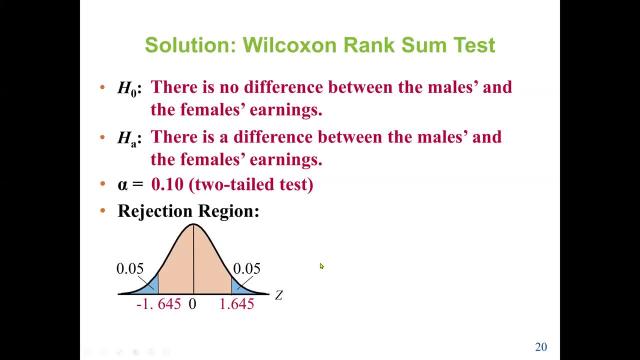 is only the alpha, Because it will be Z one minus alpha over two. So you plug in the alpha: one minus 0.10 over two. Whatever value you get, you go to the Z table and look for it And here, since we are doing two tail tests, we divide the alpha into two: 0.05 to the 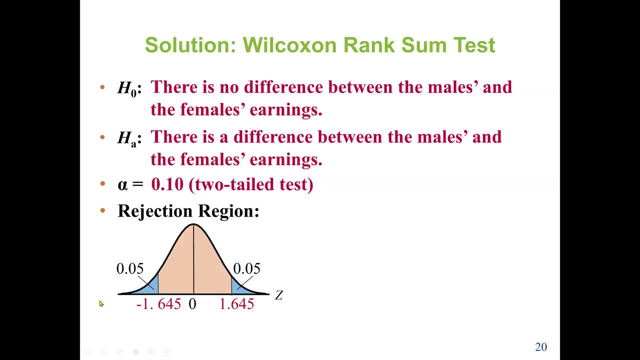 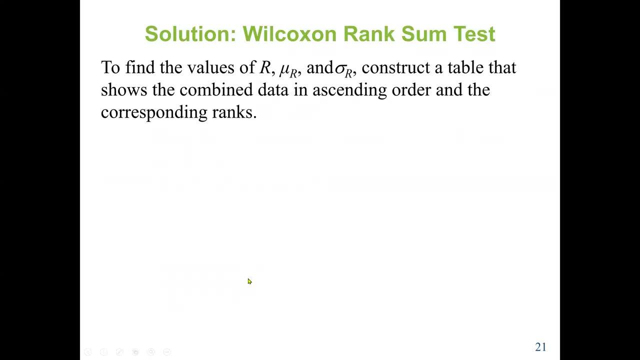 left, 0.05 to the right. So we have negative and positive. So we have negative and positive. The center will be our zero. So now we find our critical value. We want to do our test. that it is, but in order to, 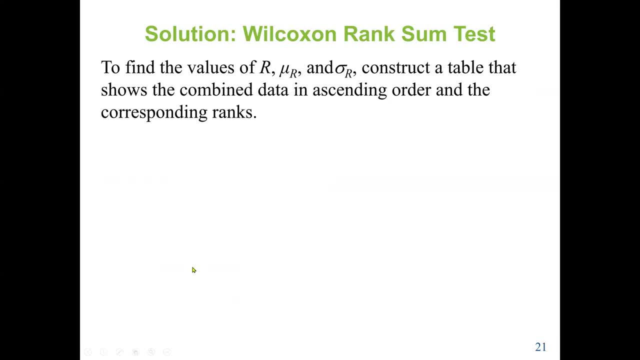 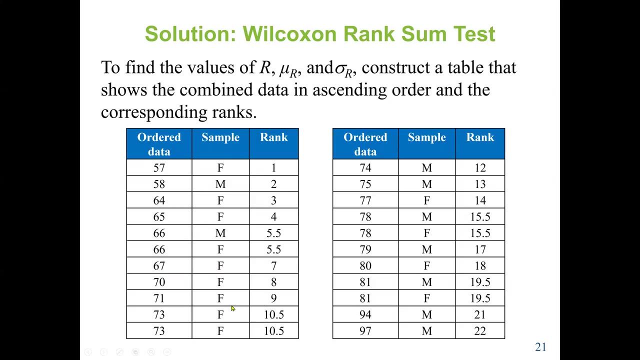 do the test that it is. we saw the formula. We need the value of R, We need the value of mu R, We need the value of standard deviation, R. So, in order to do this, we construct a table that show the combined data in ascending order, And ascending order means from the lowest. 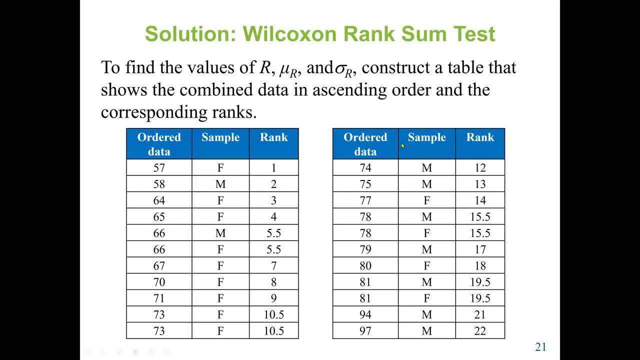 to the highest. So we look at our data. you can see that male, female, everything is mixed Because we are looking at. the lowest value in the data was 57. And that starts with the female. We rank it as one. The next value is 58. That was a male. We rank as number. 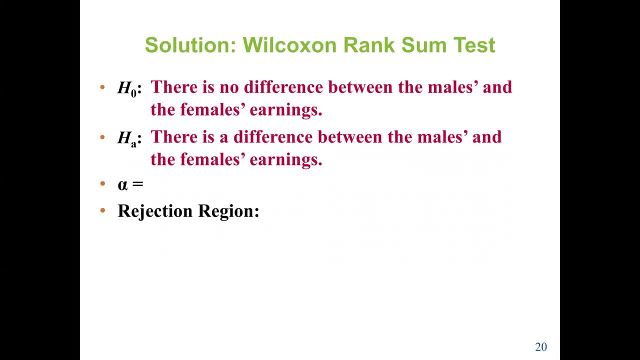 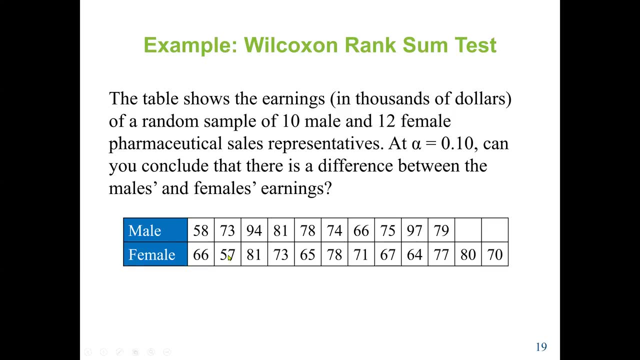 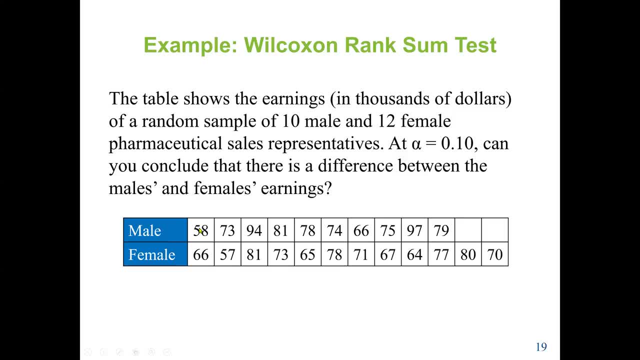 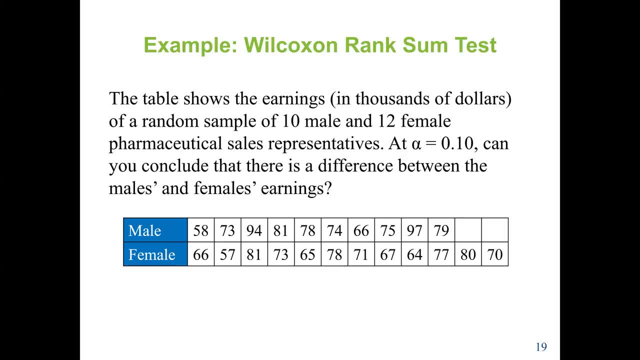 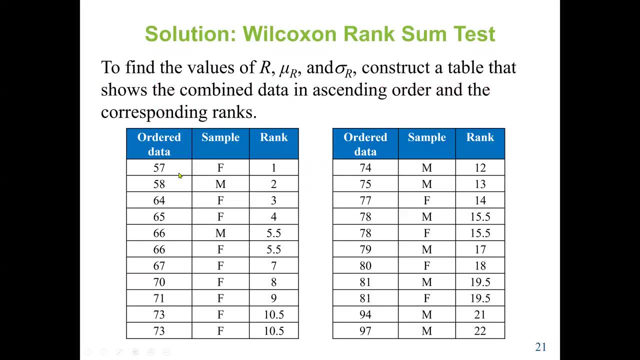 And then this will be less if we are 59. If no 59,, then we look at 60,, 61. And we keep going. So that's what we do: We combine both female and male And we rank everything. 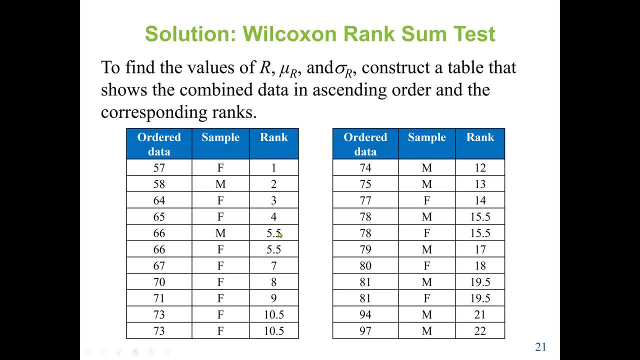 Sometimes we may have 0.5.. As we saw earlier, 0.5 means we have the same value twice. So you can see 57 was 1,, 58 was 2.. 64 is only 1.. Then we will add this value twice. So 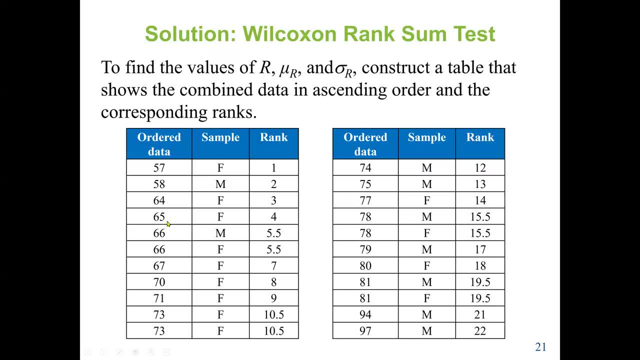 Z is 1.. Then you can see it is 50 more, And then you have 50 more. We need to calculate. it is only one, female was three, 65, female again four, but 66. we have one and two. so instead of saying: 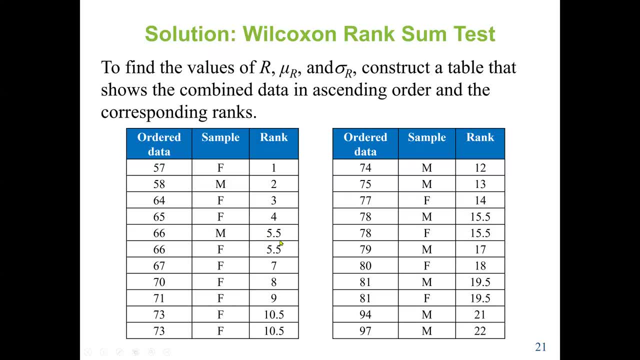 66, five, another 66, so we say 5.5 each, then we go to 67. it's only one, so seven, then eight, nine. seventy three is two, so ten point five. ten point five, seventy four is only one, so twelve, then thirteen, fourteen. seventy eight is two. fifteen point five, fifty point five, we skipped. 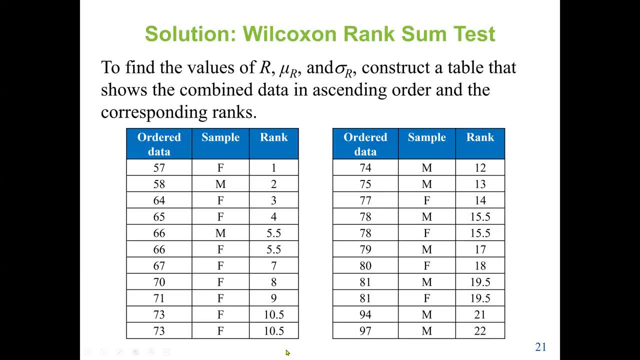 sixteen disorder. next would be seventy. you can see that anytime we have point five, we skip the next, because supposed to be five and six, but we say 0.5.5. so next to be seven, we go here nine. the net should be 10, 11.. but since they are the 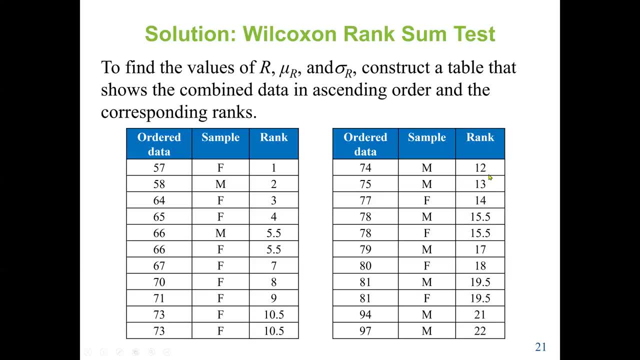 We have 10.5,, 10.5,, so the males should be 12.. So we rank it up to the end of it. The highest value was 97,, which is male, and it's only one value, so it's 22.. 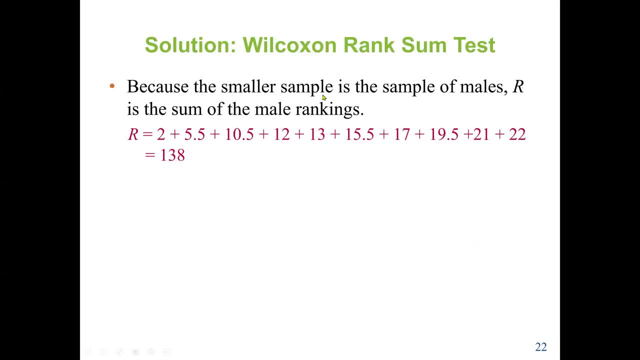 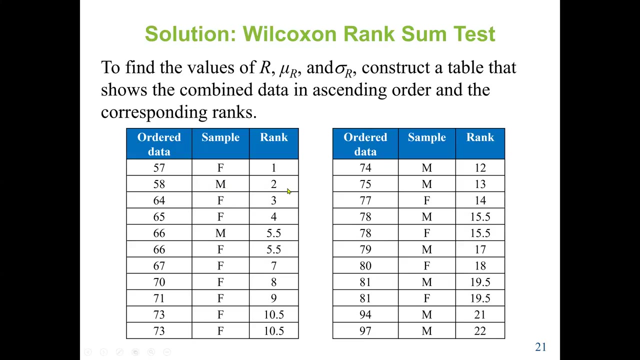 So if we know this, we are going to, because the smaller sample is the sample of males. most of the smaller sample is the sample of males. R is the sample of the male rankings. So we had all the male. so we start with the male: 2, 5.5, 2 plus 5.5, plus 12, plus. 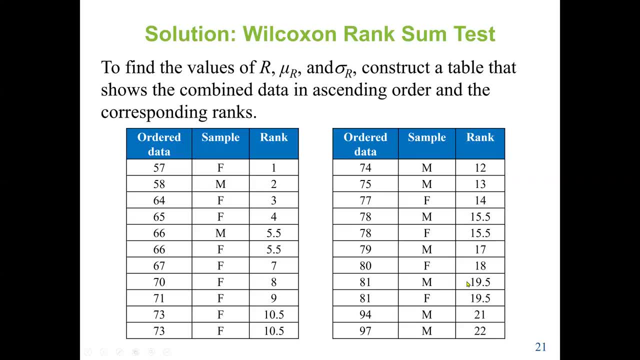 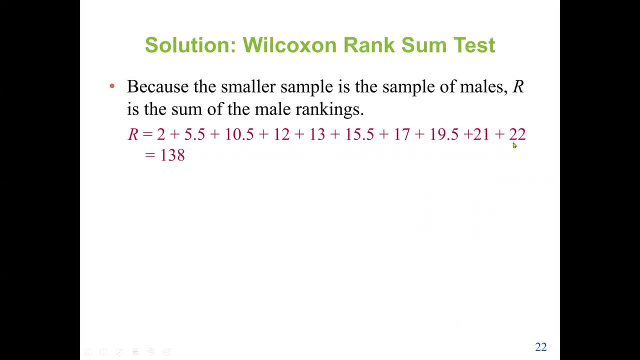 13, plus 15.5,, plus 17,, plus 19.5,, plus 21, plus 22.. And that's what we had here: 21,, 22,, 19.5.. So that will give us the R value. 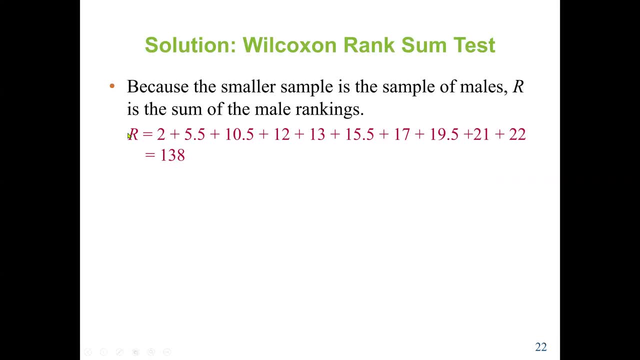 Now, we didn't add a female because it's a large sample. We said: because the smaller sample is the sample of males. R is the sum of the male ranking. Remember this when we look at the original data, which I didn't mention, but when we 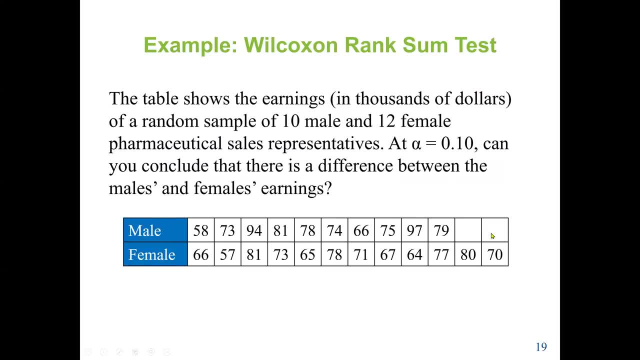 reach. look, we can see that male have two less sample, So 1, 2,, 3,, 4,, 5,, 6,, 7,, 8, 9.. So male have 10 samples values, while female has 12.. 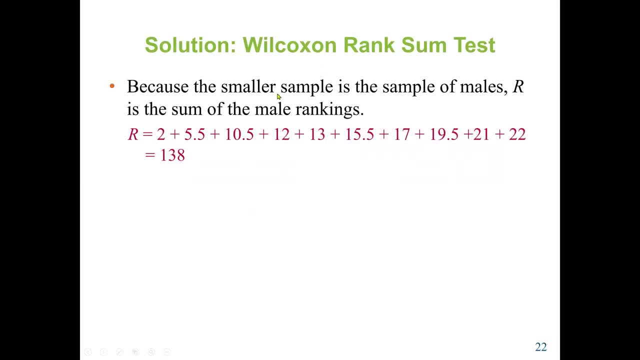 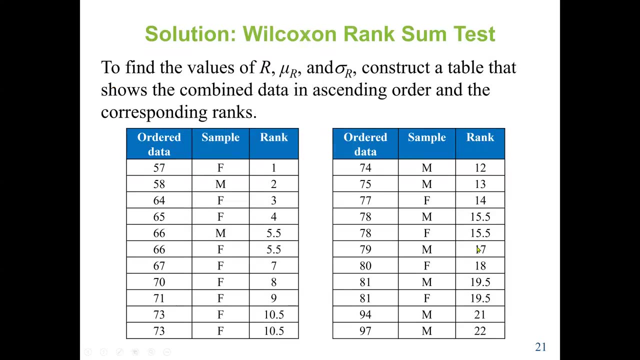 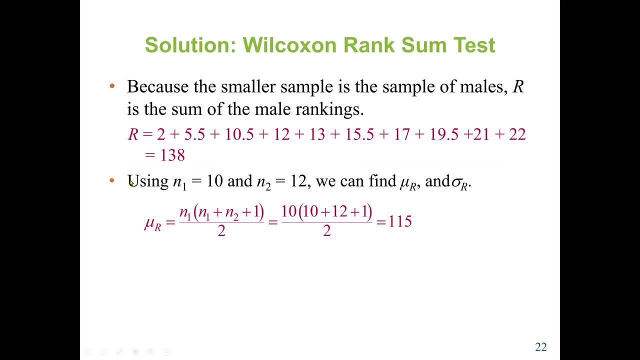 Okay, So that's what they are telling us, because the smaller sample is the sample of male. The R will be the sum of all the male rankings, So all the rankings for the male and all the sets. So next we look for N1,. N1 will be our first sample for the male, which is 10, N2 will. 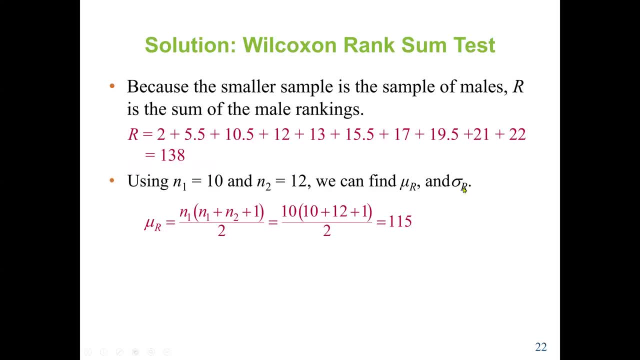 be 12.. Then we can find MR and standard deviation R, because we are going to use N1, N2 in the formula. So M mu R will be N1, parentheses- N1 plus N2 plus 1 divided by 2.. 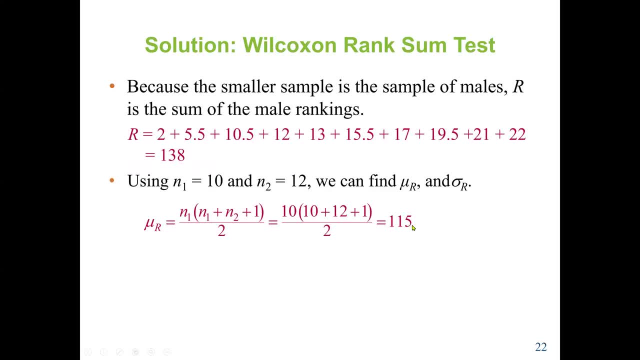 And that will give us 1 and 15,, 115.. Then we find the standard deviation which is the square root of N1 times N2.. Then N1 plus N2 plus N3, in parentheses, over 12.. We plug in the value, we do our arithmetic operation here we get 15.17.. 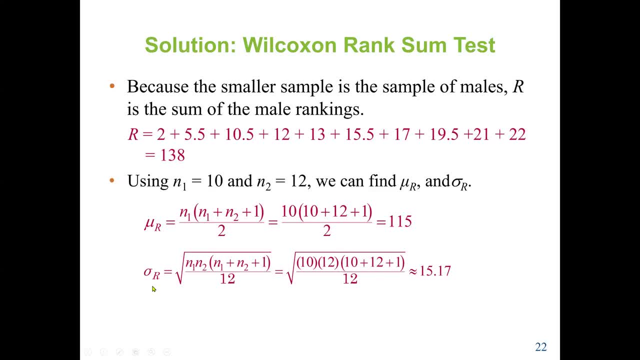 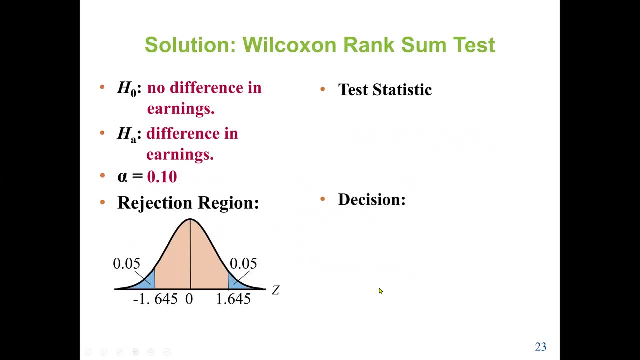 Now we know the mu R, We know the N1.. We know the standard deviation R or sigma R, and also we know the uppercase R. So if that is the case, we can find the test statistics. So Z will give me R minus mu R over standard deviation R, which will give me 1.52.. 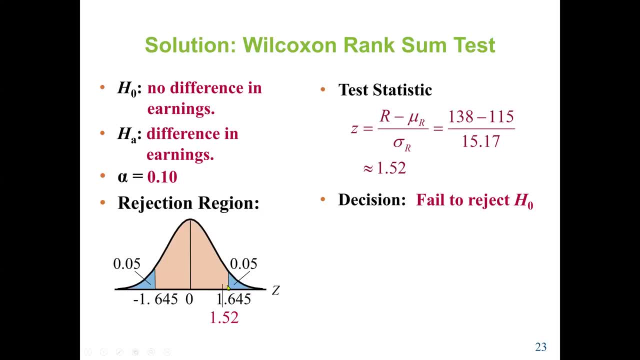 Now, when we look at the rejection regime, 1.52 fall in the brown section, which means a set. So we say our decision is failed to reject. The rejection regime will be the blue area, that's the rejection for HO. So here we say: at a 10% level of significance you cannot conclude that there is a difference.